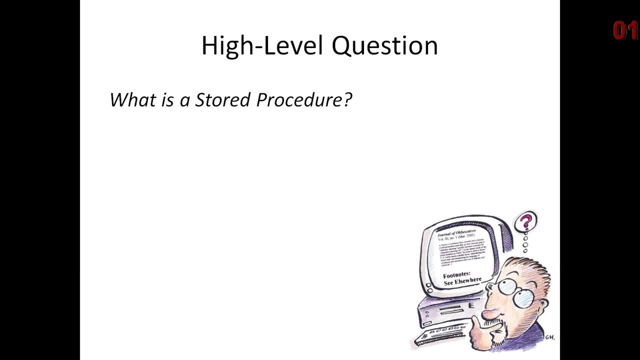 We're probably going to want to have professionals that spend a lot of time figuring out what the exact code needs to be. We only want to write that one time. We test it, we vet it, we make sure that it works and then we leave it alone. 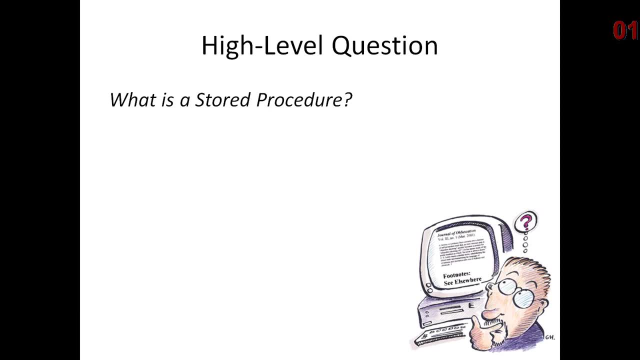 We only call it when we need it. We don't actually have to reprogram it, We don't have to change it, We don't have to code it from scratch every time we need to use it. We build it once and then save it. 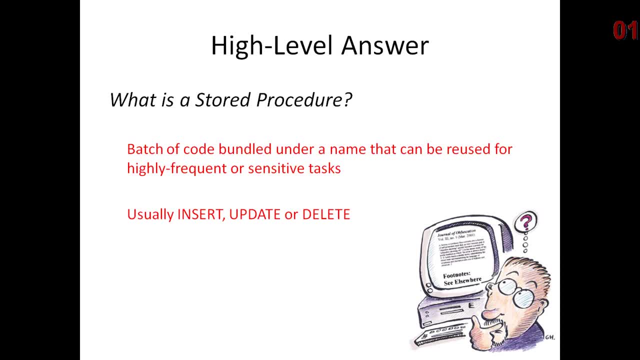 Save it, Name the object that we can reuse. So the answer I come up with when I am asked what is a stored procedure? Well, it's a batch of code. A batch of code bundled under a name that we can reuse it. 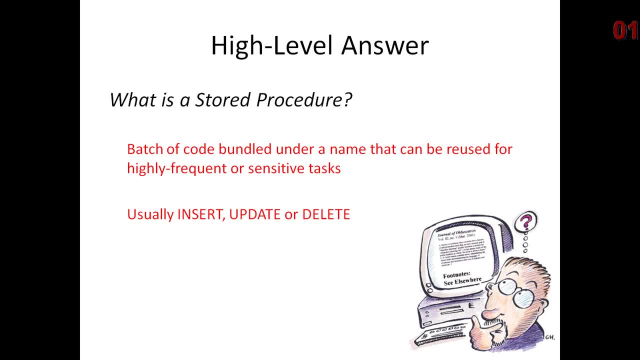 So any insert, update and delete statement. Now remember these are destructive. These can actually modify the data, Most often in a very good way. If it's not done correctly, it's a bad way. So we want to make sure that if we 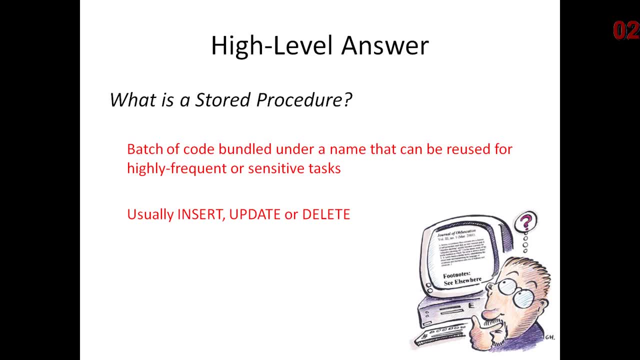 If we are potentially issuing destructive language. this is like running with scissors. We want to have professionals running with scissors. Not that you can't get hurt- You can. But if it's done by professionals we have a higher probability of it not cutting someone the way it. 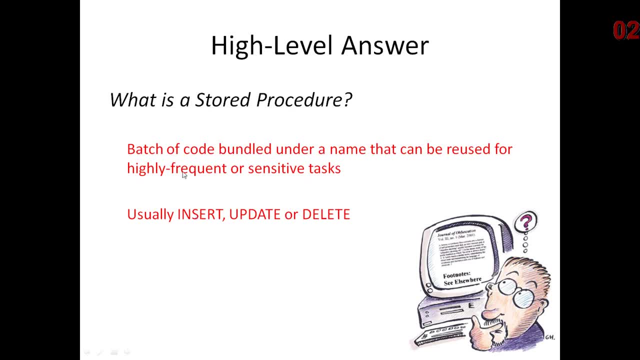 Never mind Moving forward. We have anything that is highly frequent or highly sensitive. Highly frequent would be anything, Insert any transaction that is being sold, let's say, by Amazon. They have tons of stored procedures that will manage their checkout process. 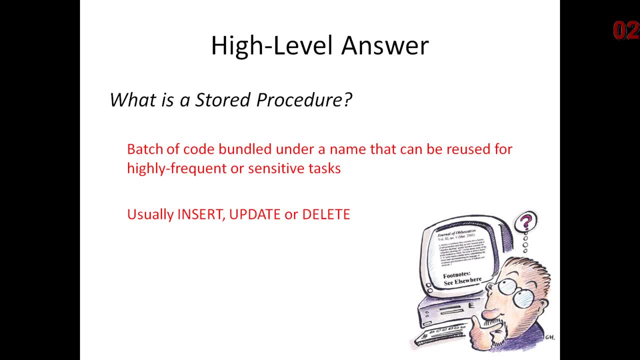 Again, highly frequent or highly sensitive, Anything involving money, Anything involving obligations for business rules, Business tasks. We want to make sure that we have code that we believe in. We don't want to have people winging it every time we need to do a sale. 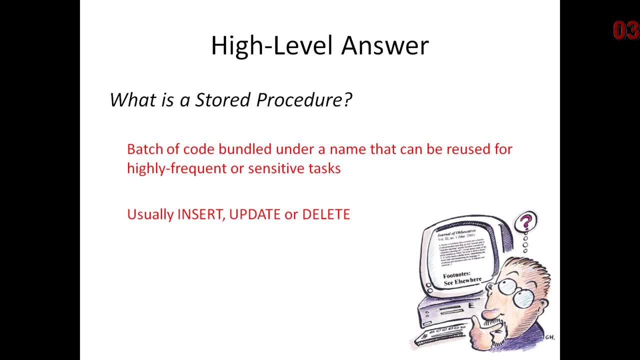 We want to Code what the sale looks like Or the order. What does it look like? What does it need to do? What are all the checks and balances? What are all of the business rules that need to be evaluated? Write that one time. 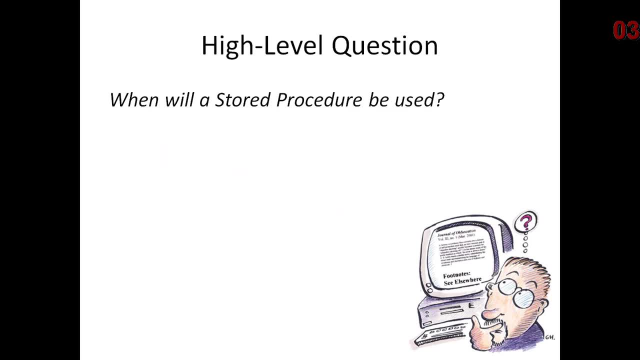 And then save it. call it whenever we need to issue a sale- Pretty simple. When will it be used? Let's take a closer look. Highly frequent tasks, such as authentication When we log into Facebook or MSN Live Passport- What actually is happening? 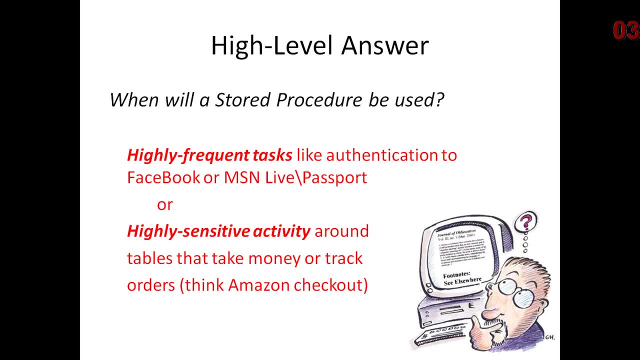 While we present a user ID with a password, it actually a stored procedure will take those two pieces of information and go check in a database somewhere. That is like, hey yo, I got a user ID. this Is this the password you have stored. 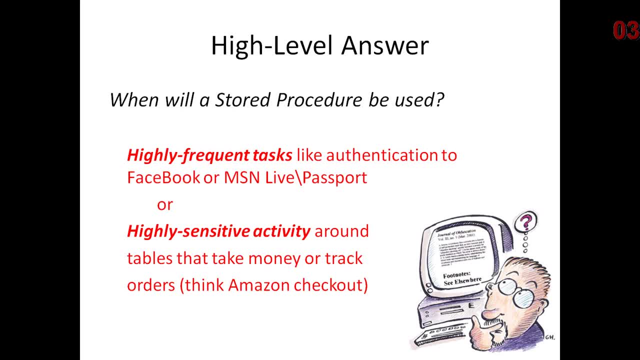 Yes or no. Oh, it is Great. Well, let's let them in So highly frequent, Not a dozen times a day, But think of hundreds of millions of times a day, And it really honestly doesn't have to be hundreds of millions. 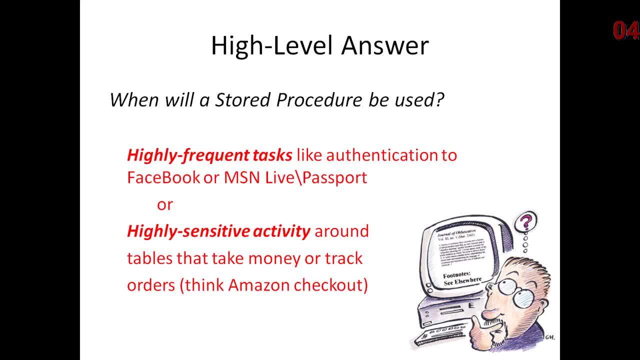 It could theoretically be a dozen times a day that we would still want to have a stored procedure handling those tasks Anytime. we don't want to recode Anytime. it's an exact duplicate. Now the actual data may change. The product that is ordered, for example, in Amazon Checkout, might be different. 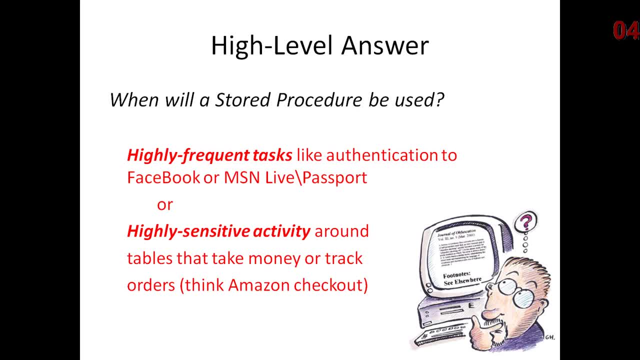 Last week we ordered a lawnmower. Now we're ordering a set of golf clubs. Not that you'd buy golf clubs from Amazon, but let's just say you did. What is changing is only the product ID, The actual process of checking for business rules, valid credit card information, looking for any outstanding red flags- all of that is the same. 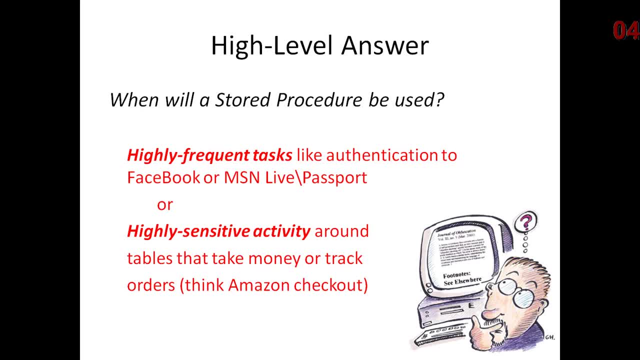 All we need to do is update the vehicle that is going to go to the database with new Data, new passengers that are going to be in that vehicle, Highly sensitive again, anything that tracks money, anything that tracks orders, Simply because we want to make sure that, if we're going to engage in a business obligation, there's now a service or a product that is expected somewhere. 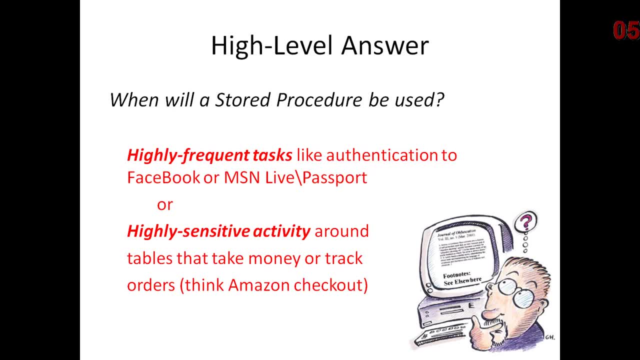 We want to do it right And again, we don't tend to survive well if we wing it. every single solitary time we engage in a business transaction, We want to do it right, We want to do it correctly And we spend many hours making sure that the process is done correctly. 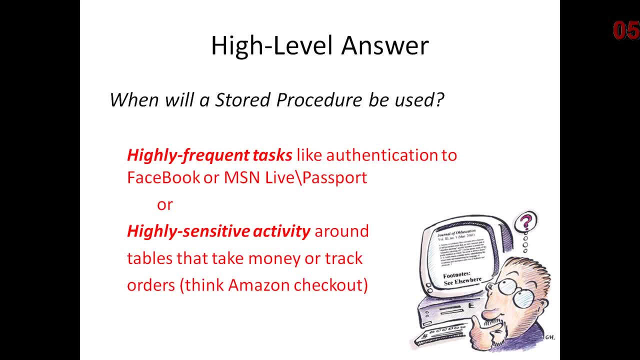 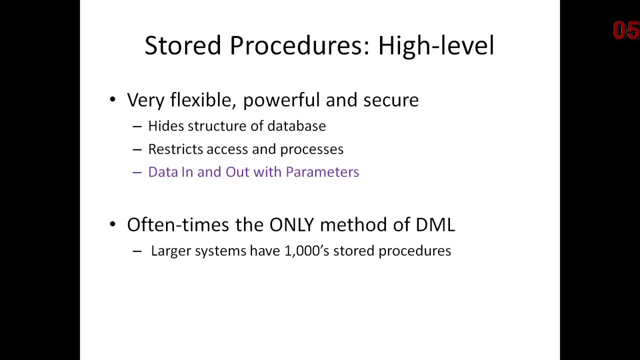 Once we code that we want to put that baby to bed so it doesn't wake up anymore, And that's how we use stored procedures. Lecture's over, Just kidding. We have several ways to make a stored procedure very flexible, Assuming it's very flexible, very powerful and secure. 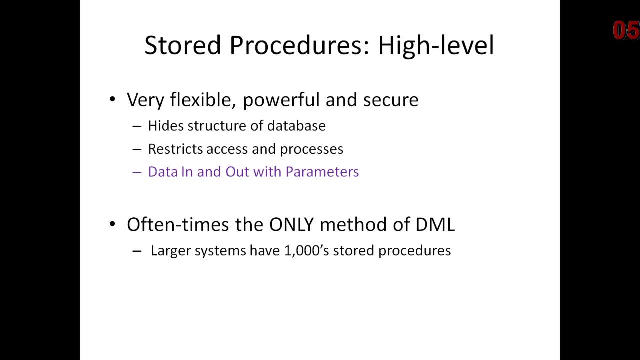 Why Well, We're hiding the structure of the database. The code to go do an order is not as visible to the application as if they had to issue the exact code. Imagine for a brief second if we didn't have stored procedures. we would have to code essentially all the insert, update, delete. from where statement? 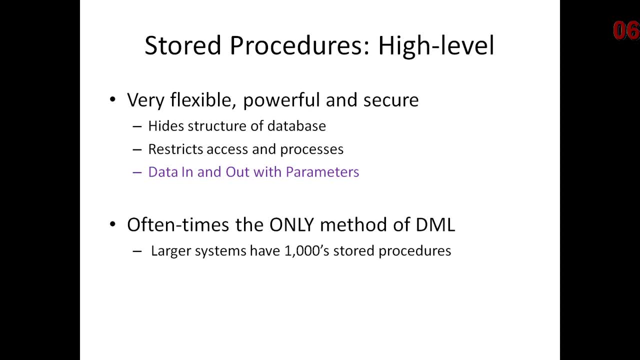 Yes, Each time we wanted to issue the same activity, So we would have to be aware of where the data lives, What are the table names, What are the sensitive business rules. If we code it and then save it as a stored procedure, all of that is now invisible. 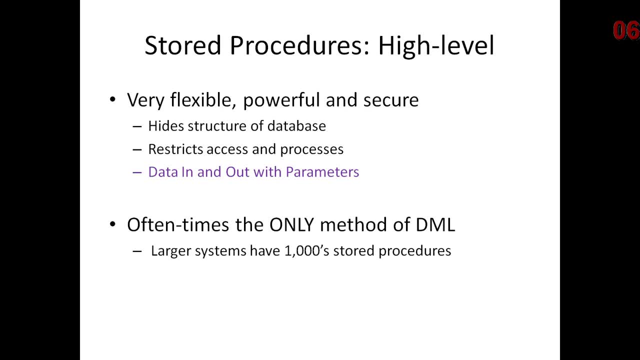 We don't have to actually have that code living in the application. We just call a stored procedure by name. You can call it Dave And give it the new data that has to be transported with that store procedure and it takes care of it. 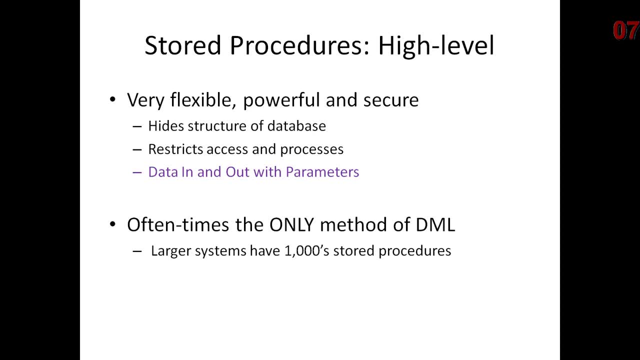 So it's a layer of security when we don't have to open up the structure of the database for the application to see. All we need to know is the name of the stored procedure. Again, it increases security with restricting access and processes. People have to know exactly what the stored procedure is and if they don't have permissions. 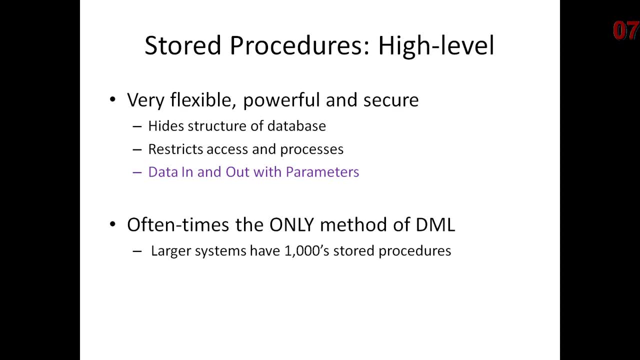 They can't call it. So even if they do know the name of it, they still have to be given explicit permissions to operate that vehicle, to leverage that stored procedure. So we're gaining security. I put in purple here data in and out with parameters. 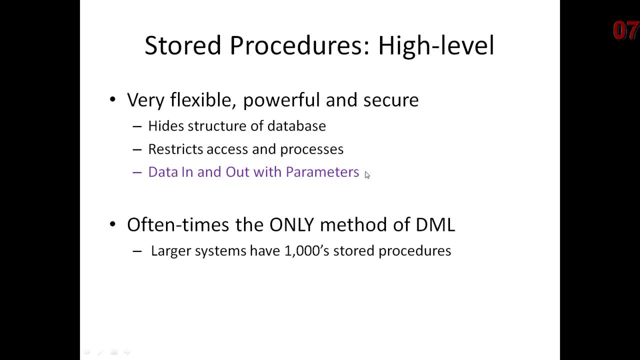 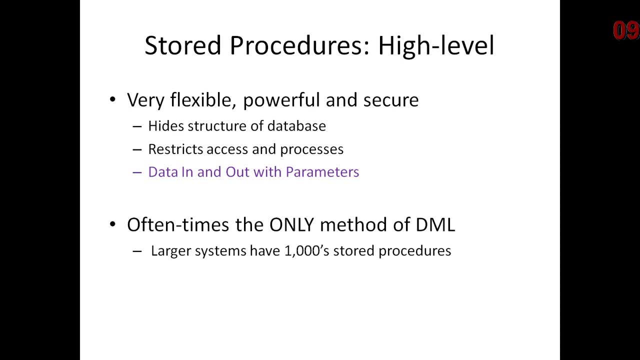 So if we are ordering products and we're expecting a product name, the stored procedure is going to be the new data. difficult to have people coding orders even if all we were doing is clicking on menus. it doesn't scale. we have to have methods to scale to increase the volume. 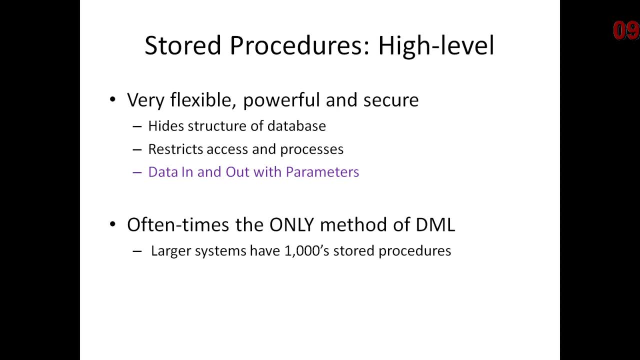 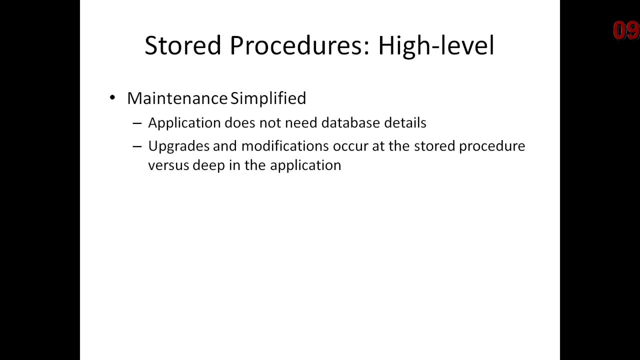 and we do that through code saved code. we can simplify our maintenance. these are advantages of store procedures. the application doesn't need to know the database details. as I mentioned, that's a security feature, but it's also allowing us to make changes without impacting the application. in the old days, we had to 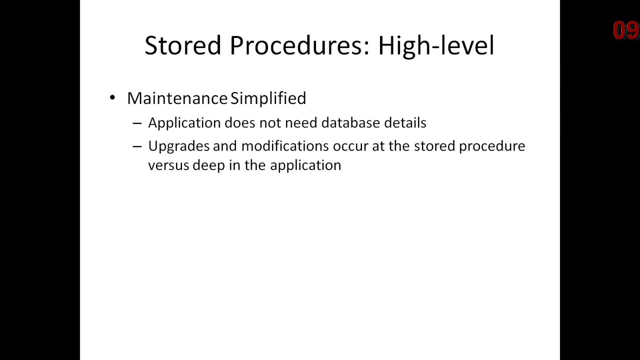 hard code the file locations of data within the application. so if we moved the file in a hard drive of where the data was actually stored, we would have to update the application. that was not only cumbersome, it opened up the opportunity for errors and it it didn't always go well, because we didn't always 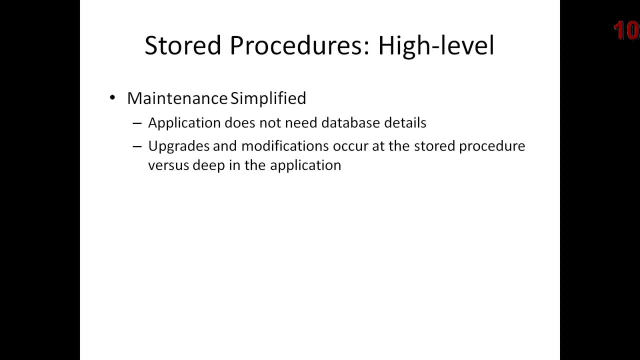 know where you see the location of the files was included in the application, so we changed it. once application breaks and we have to search through hundreds of thousands, if not millions, of lines of code trying to find where else is the physical location of this data specified. so again, having store procedures is one. 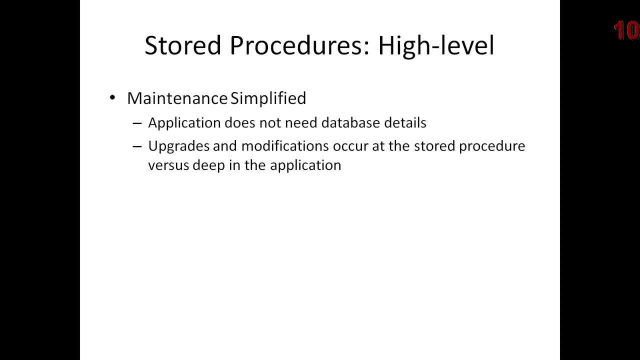 more layer of abstraction not only does it make the data more secure but it also removes the application from having to know the details of the application and exactly to where the data � Zombies isblick rozm Themeplay does that mean we can make those modifications happen way faster by 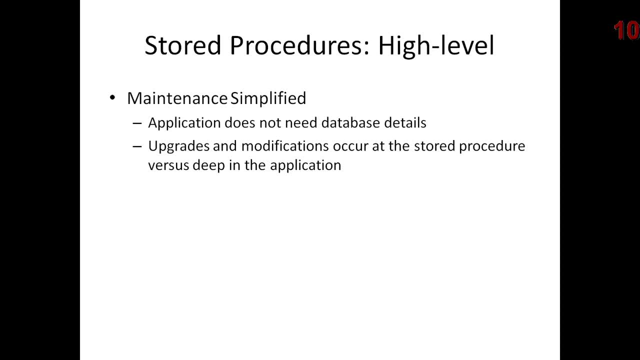 changing the application leaves the application where data is located in a database. Upgrades and modifications can occur at the store procedure. let layer within the database. if we change store procedure, enter the application, we can change the code. we don't necessarily even have to have access to the base tables as long as we 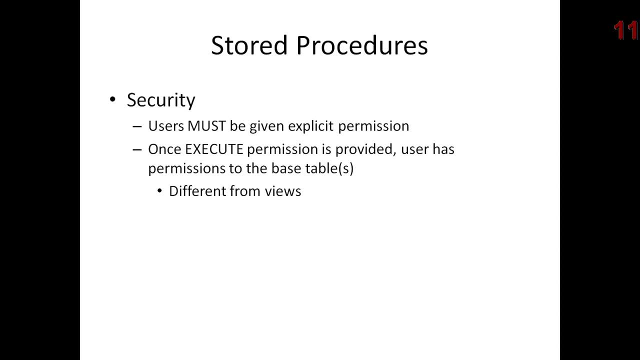 have execute permission to the store procedure, we can issue the commands that are included within the store procedure touching certain objects that might not otherwise have been given explicit permission to our to ourselves. I put down that this is different than views. even with views, we have to have access. 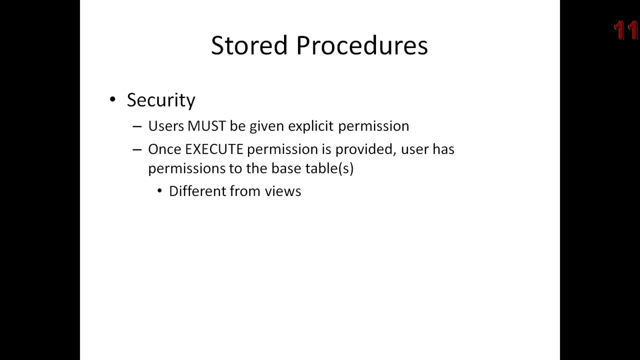 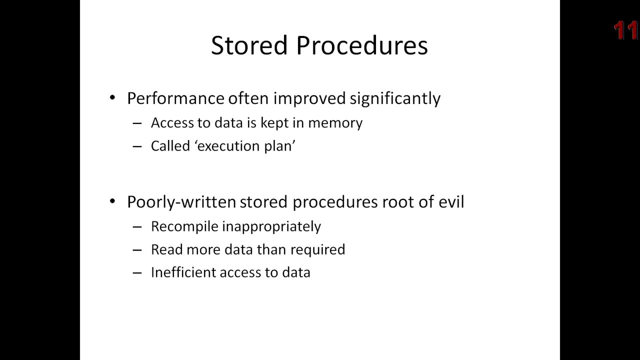 to the base table that underlies where the data comes from. in a view moving forward, we can gain significant, significant performance improvement with store procedures for one reason only: the execution plan, how data is accessed- is stored in memory. so it's: imagine: going to deliver pizzas, we're going to deliver pizza. we're going to deliver pizza, we're going to. 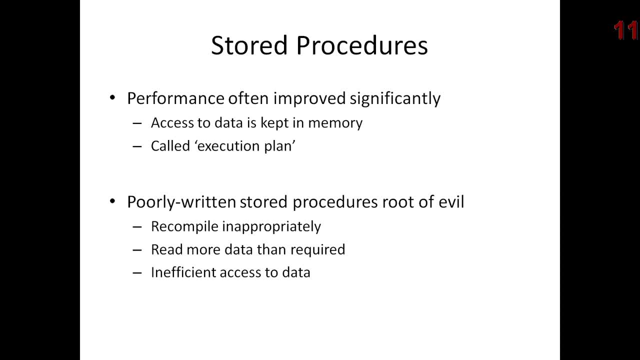 have a pizza theme here. stay with me if we're delivering pizzas. in the old days we had to know this: the grid of the city, being able to look at a map and say, oh, yeah, yeah, for Northeast, 45th Street, 3815 North. okay, so we have an understanding. 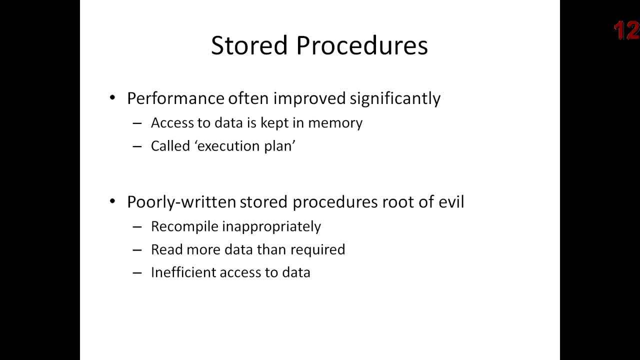 of how the grid system works in the city. well, now we have directions. imagine having to load the directions to deliver a pizza. in this case, we're delivering data to the database. we have to have a, a, an execution plan, a map, a set of directions of how to get to the data. 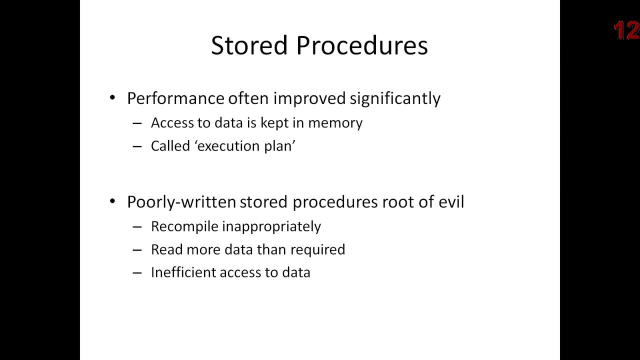 which indexes are we going to use? are we going to scan data? are we going to use an index? are we going to have an a lot of matches of for joining tables, or are we not? all of this is compiled one time when the store procedure is used, when its 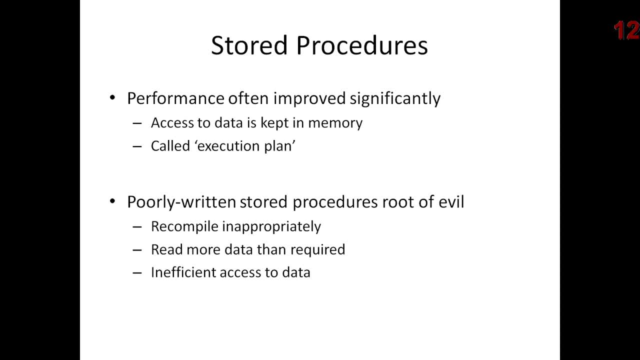 first run, the very first time it is run, it compiles an execution plan and that stays in memory. hopefully it stays in memory. there's there's reasons why that it will fall out of memory, but we will not get into that in this lecture. we don't have to compile the execution plan whenever we call the code. it is already. 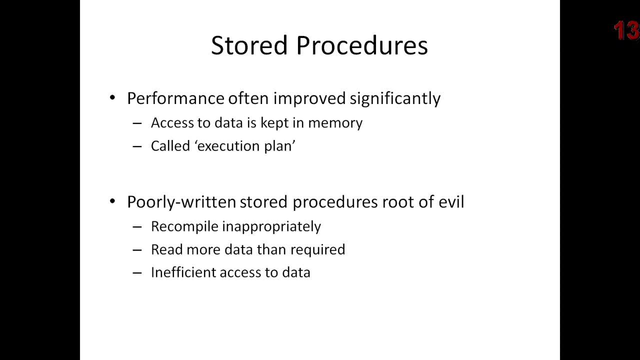 in memory. the first question might be: so what well? assume that if a store procedures called 50,000 times a minute because we're selling 50,000 items a minute before Amazon to have to recompile the access to the data 50,000? 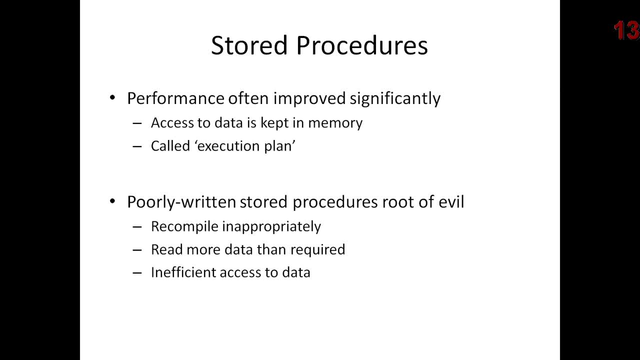 times is not only a waste of time but it's it's prohibitive, it is exp. it is. it would slow down the system to a crawl. we would not be able to process 50,000 sales a minute because we'd be spending the majority of the time reassembling, recompiling the 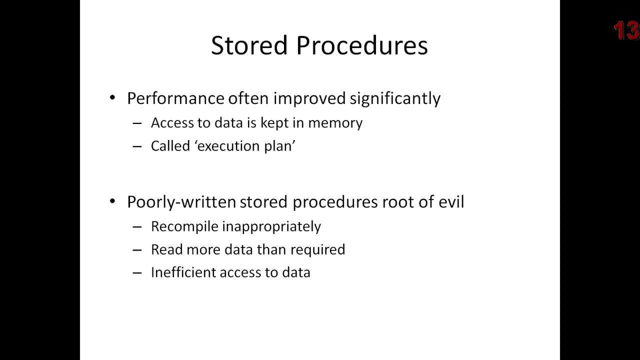 method that we're going to get to the data. if we ever do see- and we'll learn about this in our optimization and tuning module- if we ever do see- a high amount of CPU, sometimes it's due to a poorly written stored procedure that is causing the execution plan to be recompiled each time the store 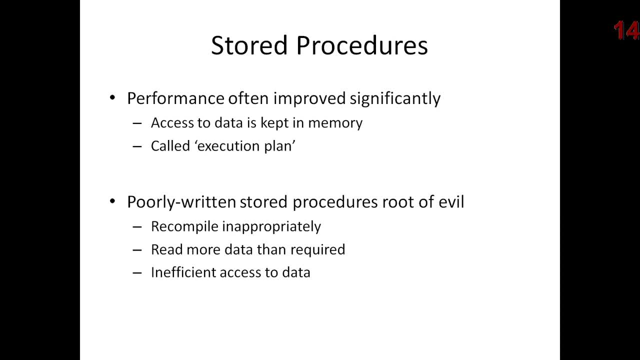 procedures called, we're defeating the entire purpose of having store procedures. if that is the case, we will learn more about that again. just because we have stored procedures doesn't mean that all as well we can. I've seen some very poorly behaving production environments, in part because 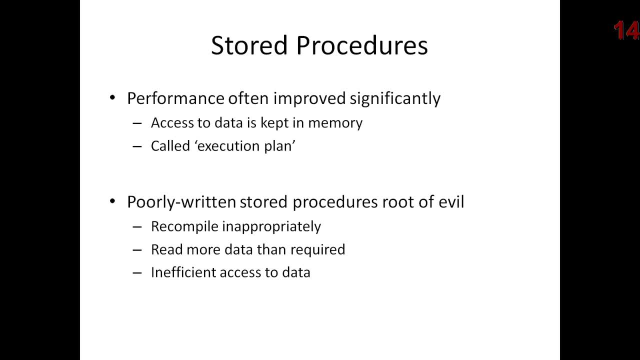 they had poorly written store procedures. sometimes people think, well, I wrote a store procedure for it, yeah, well, that that doesn't mean that it's guaranteed to run well. it still has to be well written code. just because you saved it with a name doesn't mean that it's automatically going to behave correctly, so we might be. 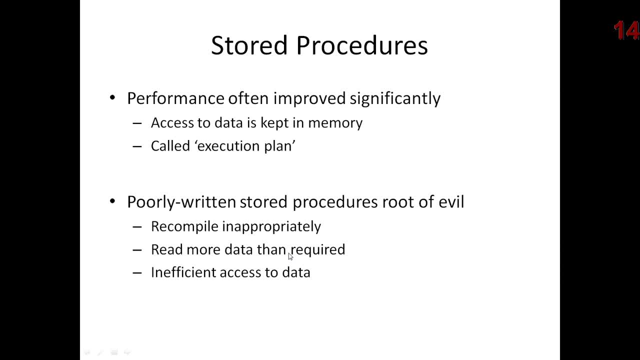 able to save recompilation? we might not. we still have to write well-defined code. we might end up reading more data than is required. we might be sorting inefficiently. we might have using the wrong it. we might be using the wrong indexes. we might be joining tables incorrectly. we might be introducing 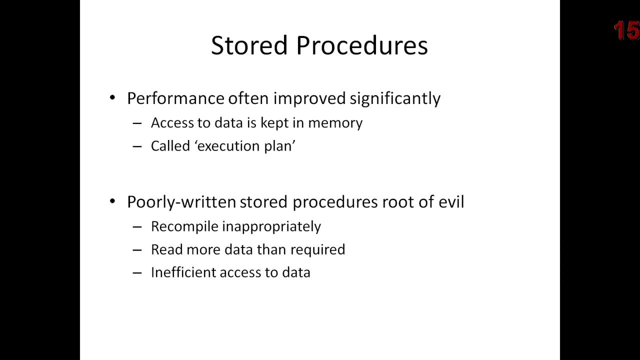 higher-level locks and what we really are within what is really required. the takeaway from this slide is: we can most often save performance. we're going to reduce the number of CPUs issued each time that we call this code. we are going to be able to access data quickly. 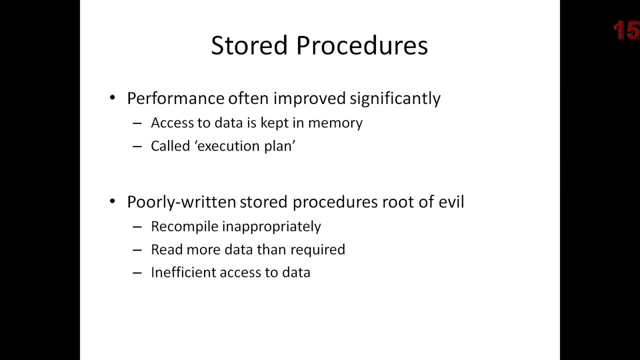 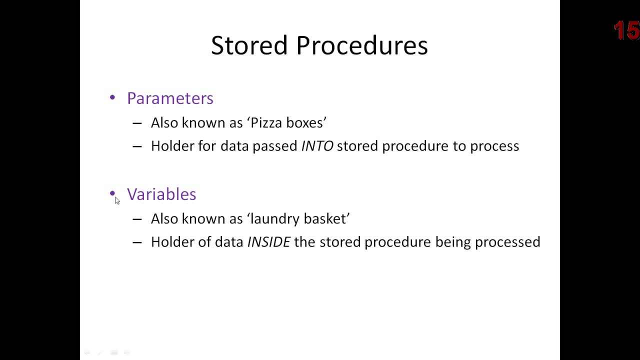 and efficiently because the system knows how to get there. but that's not guaranteed, especially if we are making mistakes and how we write. I said there was a pizza theme going here, a parameter I refer to as pizza boxes to holder for data passed from outside of the store. 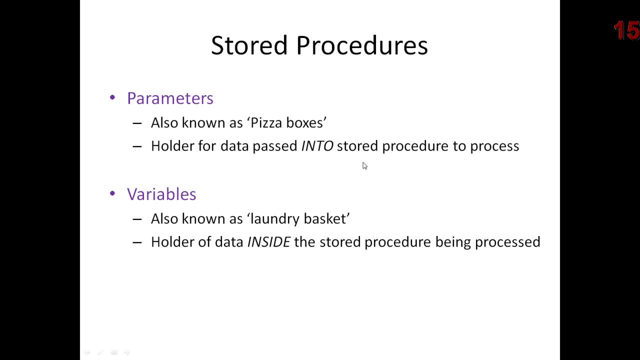 procedure into the store procedure. this is very, very common. this is how we can have perhaps a registration process for adding new students to the university and all we need is first name, last name, address, city, state, zip and then pass that to the store procedure so there might be ten parameters passed to one single store procedure when that 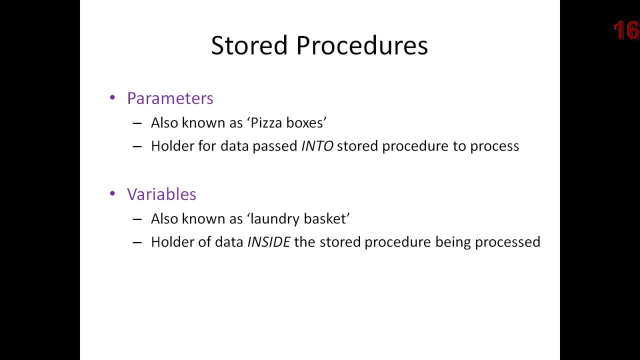 procedure is armed with pizza in pizza boxes. they can take off and deliver the data. deliver the pizza to wherever it needs to go. that is a parameter. looks exactly very similar to a parameter. is a variable. I call this a laundry basket. why is it? what's the difference? in a laundry basket is a logical answer. quite Gay, much fine, but those references are дела. 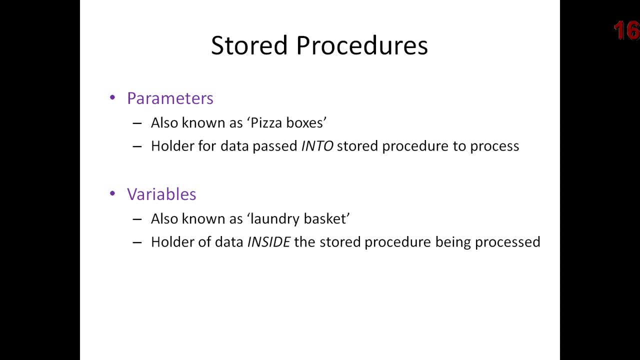 Can the bar see it? number one: perché o AI? no? The second thing we do to avoid broken minutes: get in a pizza box. well, both are vehicles, both are holders of some items. one is external, one is internal, so a variable. once we have data inside the 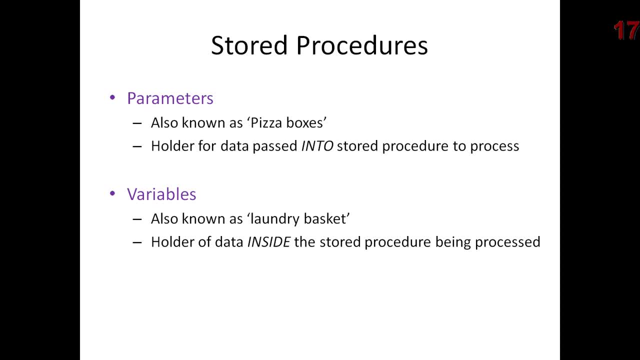 store procedure and we need to move data around. we use the same constructs that look like parameters are just used internally. so we talk about a variable and we'll see these in just a second. that is for data inside the store procedure, not introduced from outside, so an application or a web form may collect. 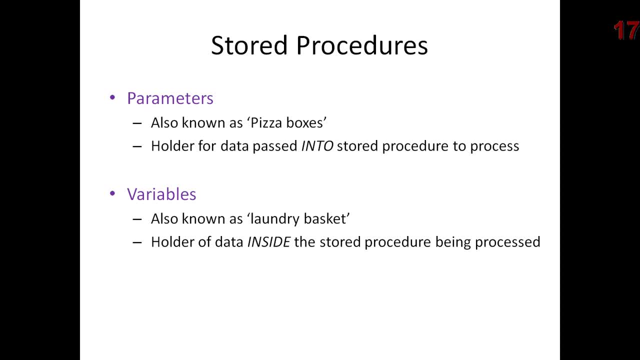 data and then pass it to a store procedure that would be used as a parameter. once we get inside and we're calculating things and we are moving data around, we're comparing against previous values. we might do the same thing, but they're referred to as variables. let's take a look at a very 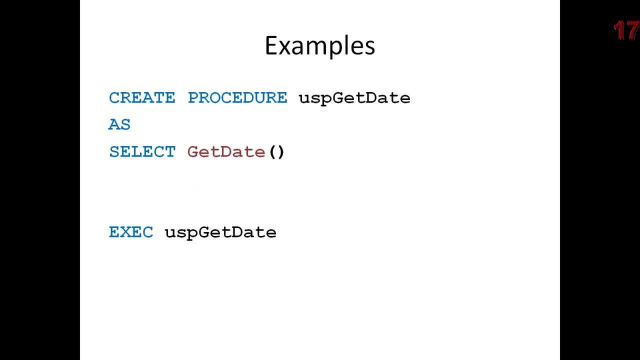 simple store procedure. this is perhaps as simple a store procedure as we can possibly get. we use the command create as we do for a table. all objects that are created within database management systems are issued with the create statement, so create space procedure. then we give it a name. in this case, USP stands for user stored. 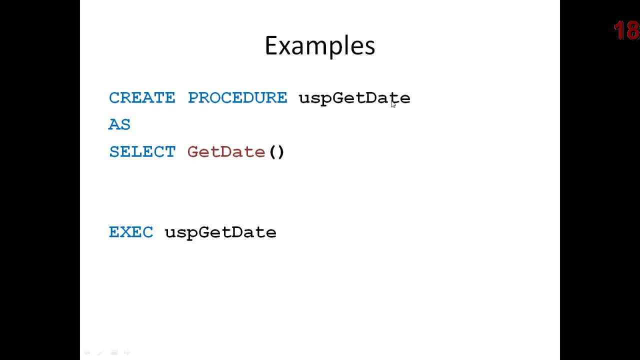 procedure. I'm calling this get date the key word, as tells the system that the next command or anything following the as is what is going to be processed. you, while this- this is a two-word store procedure- select get date. let's go out to our management system and take a closer look at this. let's create this. 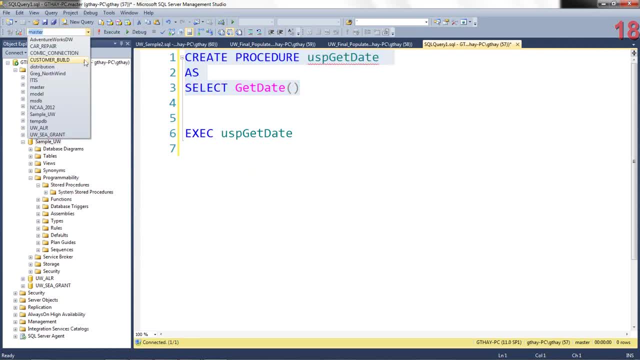 store procedure. if I'm not exactly sure, if I created. yes, go to a database that I know it doesn't exist in. we issue this command. it says okay. so we now have a store procedure called get date. what is this going to do? well, it's going to do. 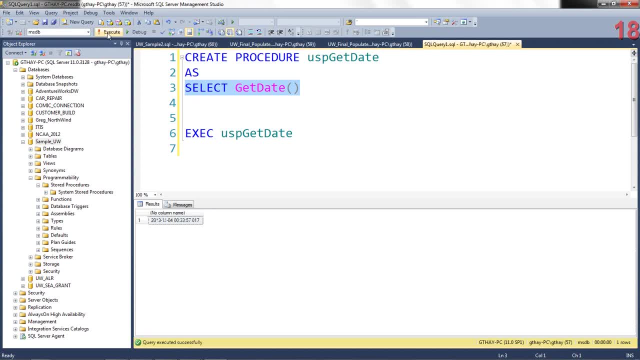 this command. so I just highlight this command and run it. it's going to go out and calculate it. as you can see it gets executed the faster it actually did. it is going to run this, of course. okay, so I can do that a thousand times, or I can just call. 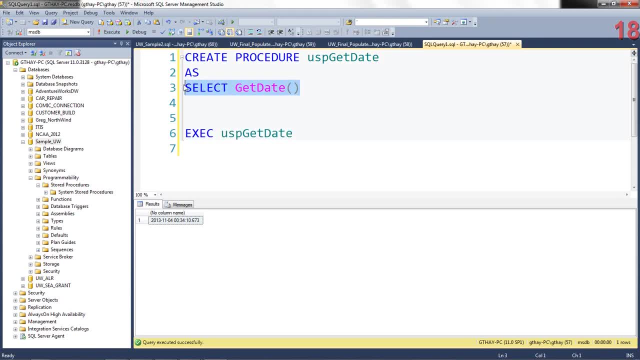 this store procedure that will then run this code. ok, now people might be saying: okay, don't think I would be gaining much if I put a stored procedure around. select get date- probably not, but imagine having I don't know lines deep And instead of having to write that 300, 400 lines each time we wanted to process 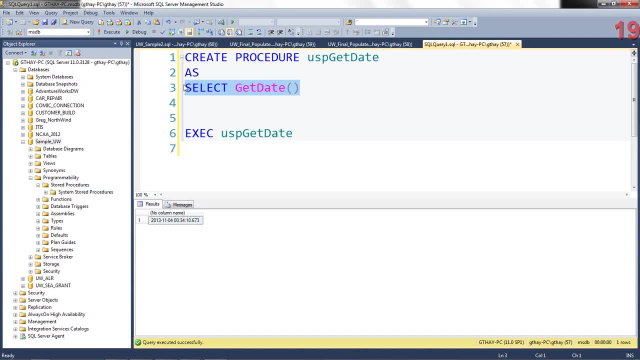 whatever it did. why not save it and just call it whenever we need it? Let's add a little bit more flexibility here. We don't have any parameters. We don't have any variables. We do have a function here: GetDate is a function. Let's modify this. So we're going to issue the alter statement. 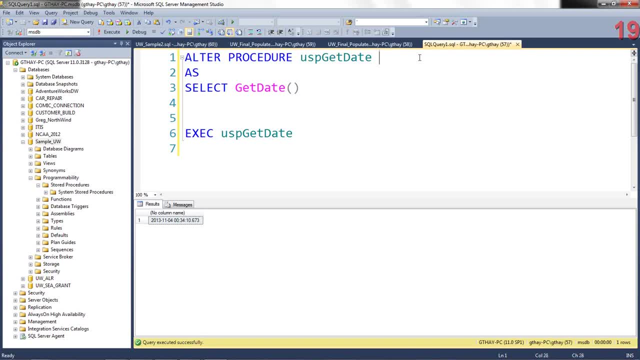 alter procedure. Now we can make some changes. How can we make this GetDate more flexible? What if we could issue GetDate but then pass in either days in the future or the number of days in the past that we want to get the date for? Okay, so let's do that. Let's put a parameter here. 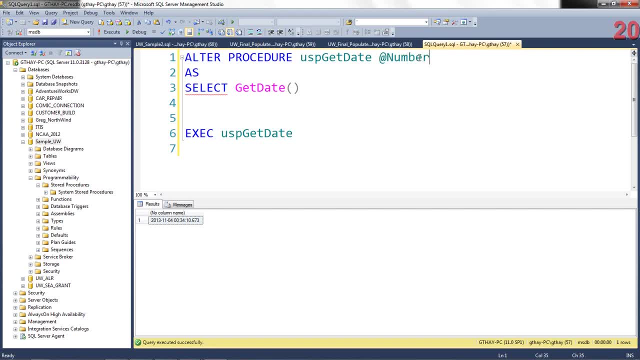 at number of days. I'm just going to make this up here. number of days: This will be an integer data type And then we will select GetDate minus- see if you can stay with me here- number of days. So, instead of having to issue this code, select GetDate and then some number. I can store the. 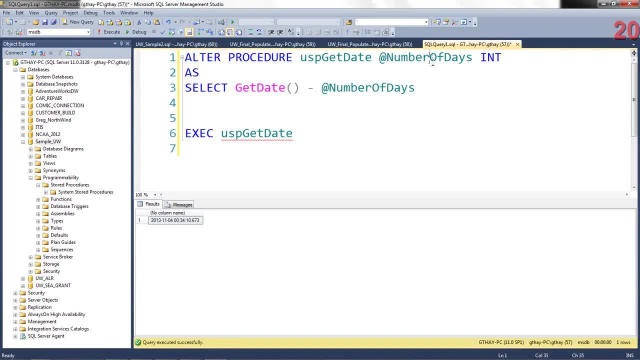 functionality of select GetDate, And it will recognize that it's going to take one parameter. So now we're going to execute this. What's our favorite number? I don't know. 11.. Oops, We don't have to put the minus sign, We just put the number 11.. Now if 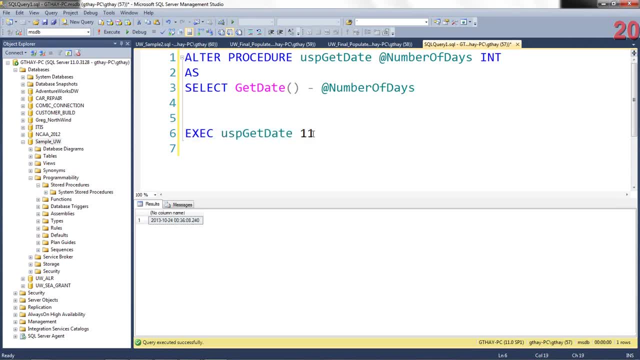 we execute this. it's going to take the 11.. It's going to take it in. It's going to put it in a pizza box. This is the pizza box. Number of days. Number of days now holds the value of 11.. 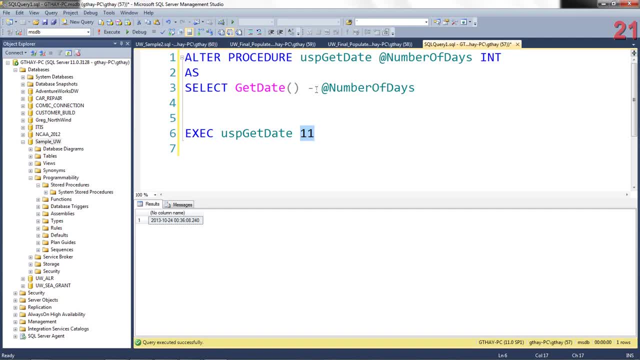 And then it processes select GetDate but take away, Okay, Whatever was in the pizza box, in this case 11.. If we look at this very closely, 11 days ago was October 24.. And this happens to be whatever time. today is 1236 AM on November. 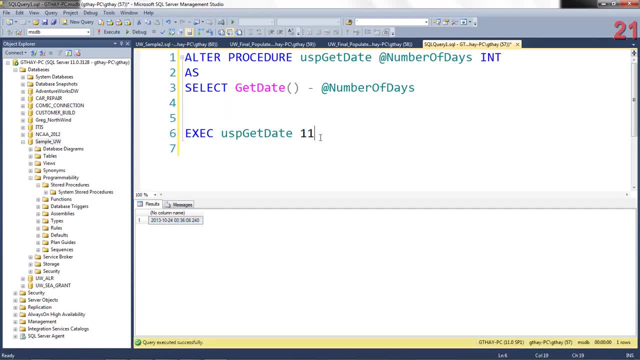 4. 11 days ago was October 24.. If I make this some large number, I don't know, 11,090.. This will go find it. It was 1983, June 25.. Okay, So now we begin to see that. okay, that might be interesting. 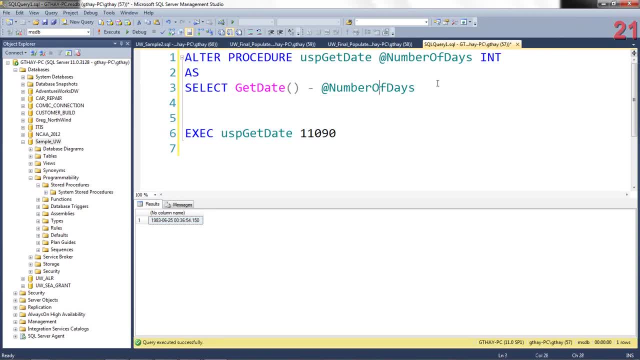 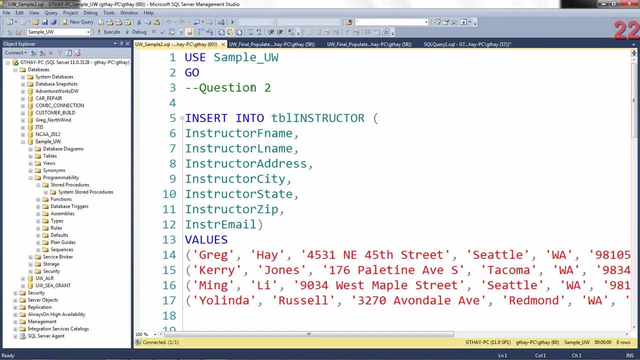 Now we're passing in a parameter And let's say we had, I don't know, another set of columns that we wanted to insert, update or delete to. Let's go see what else we have here. I have some other code And let's do. let's do this one. This is part of our lab that. 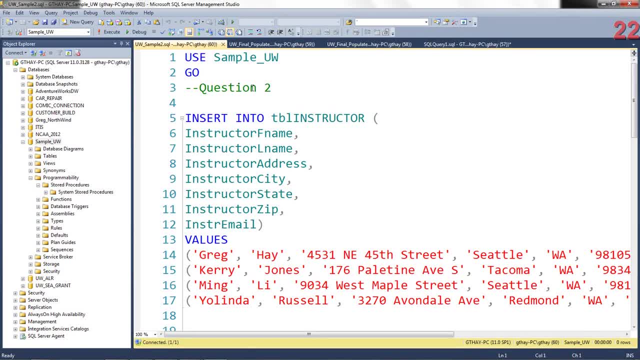 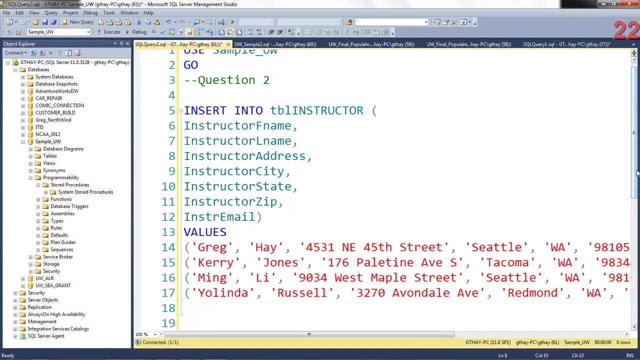 we just finished This past week. We're going to insert into TBL instructor. Okay, We hard code the columns that we want to put in, And then we have the values. Well, this kind of makes sense. Let's go ahead and copy this into a new window so we can just see it by itself. Sure, We would. 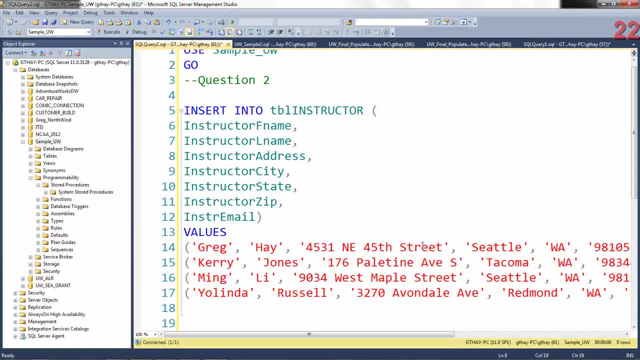 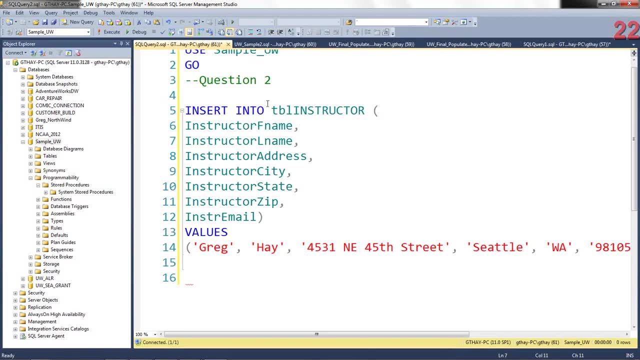 have to know and hard code these in. This is not very flexible, is what I'm trying to say. I would think if we could make these into parameters, we would begin to add value. Let's copy these. How can we take this insert statement and make it more flexible? Let's create a. 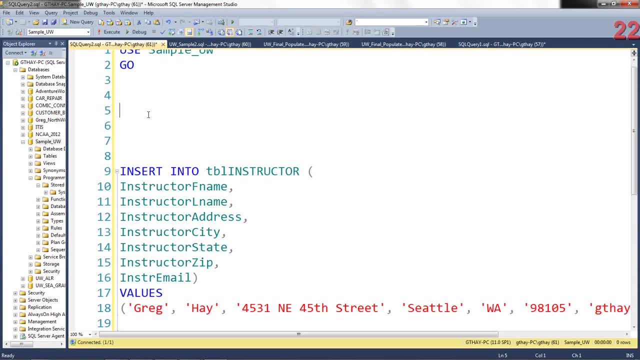 procedure around it. I have a coffee getting loose there on the table. We create a procedure. Let's give it a name USP for user store procedure. Let's go instructor insert. Let's go insert instructor. We're gonna call, we're gonna take in some parameters. This is what. 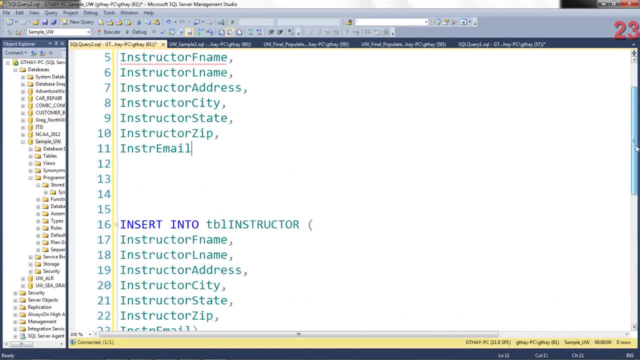 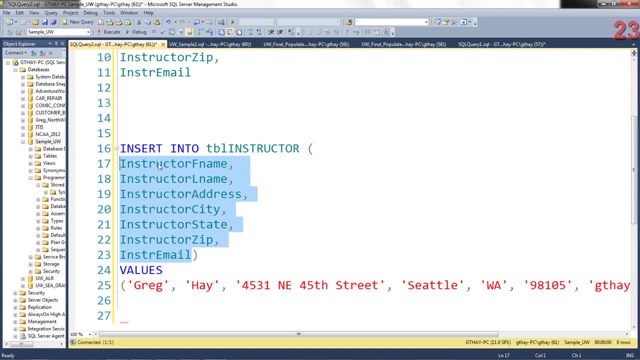 it looks like. Please notice how I just cut and pasted the columns that we want to enter. I enter values. This is our insert statement. It needs to have instructor first name, instructor last name, address, city, state, zip and email And we'll get to these values in just. 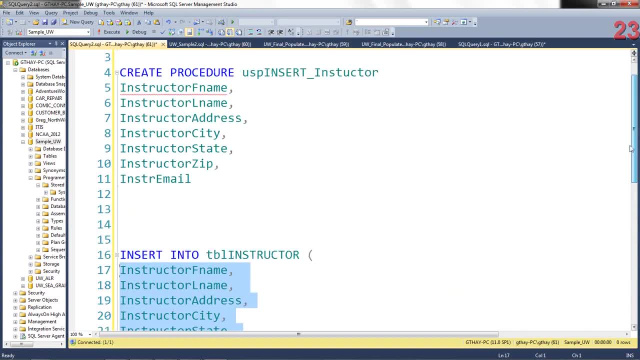 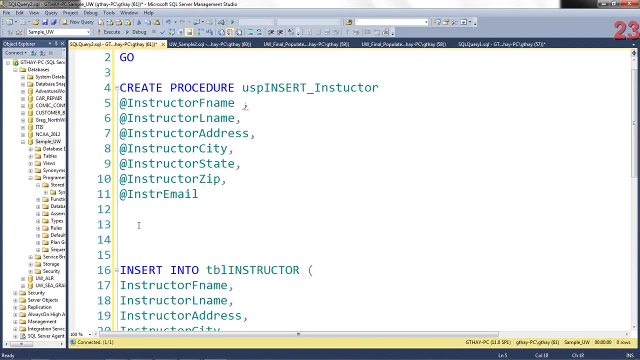 a second. I copied these, put this up here. I'm going to make each of these a parameter. Now, these are pizza boxes because they're going to take delivery of some data in. What is the data type of instructor F name? Well, we can guess or we can go look at it. So this: 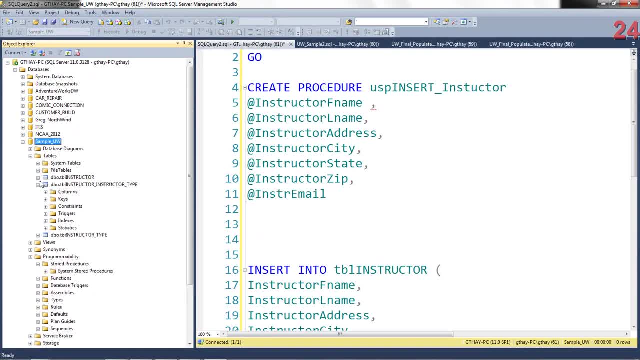 is going into TBL instructor. Let's look. Let's look at the right table: TBL instructor VARCAR45.. So this pizza box is going to take data in and it's always going to be a VARCAR45, if I spell it correctly, That's the first one. 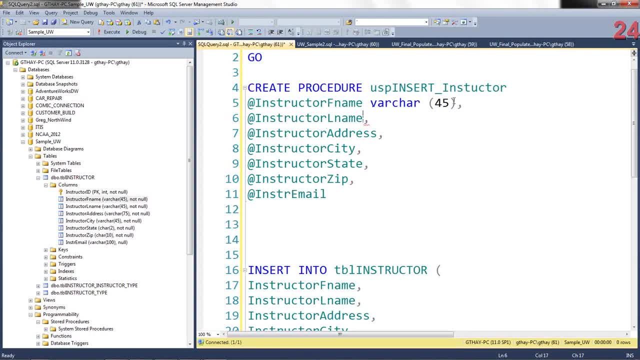 Second one. Second one is L name. That is also a VARCAR45.. I'm going to get a little bit sneaky. copy that, paste it there. Instructor address is a VARCAR75.. Instructor city is a VARCAR45.. 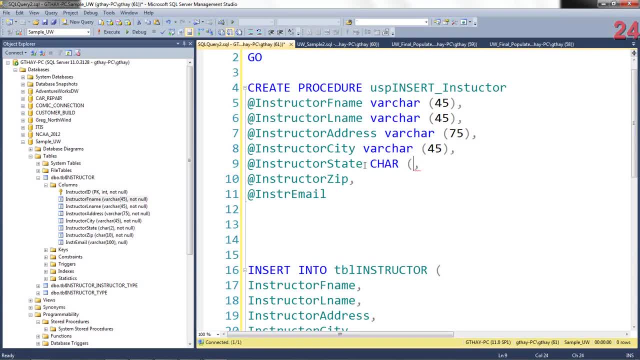 Instructor state is a character 2.. Instructor zip, I believe, is a character 10.. Instructor email is a variable 1, and then instructor e-mail is a variable character 100.. Okay, Now, all I've done is created the parameters, perhaps mapping to a web form where this: 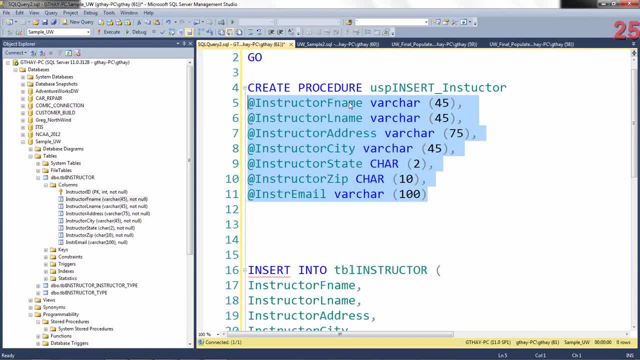 data is going to be collected whenever an instructor is hired. Key word is AS. Did you see how, before I put AS in, did you see how, before we put here, had a red line, red line? A, please, 2,, two? Did you see how, before I put thing in, we had a red line, a red line? I don't want to make this jump in. I don't want to make this jump in any further. Okay, Microsoft Word, have to BLACK ON your emails all the time and quit us now, or else this will you know, impossible to get snowing until the end. demonstrations, the parameter in my choice for done an additional. 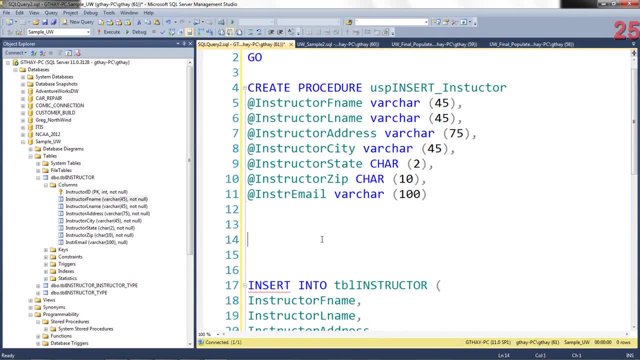 job won't be a problem to do any other way, but this is where dolls go down. So I Finished我就 pained our squiggly line right here. it's because the system is trying to tell us there's something not right immediately nearby. we put as in there. it goes away like 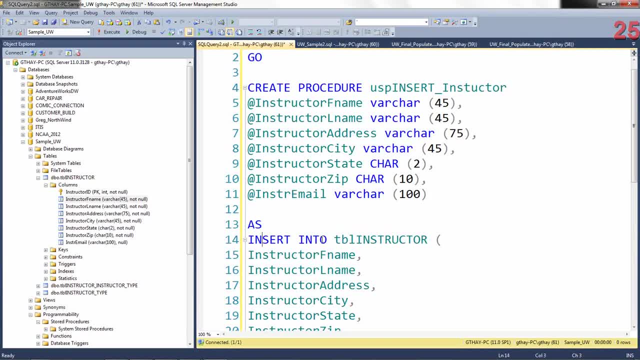 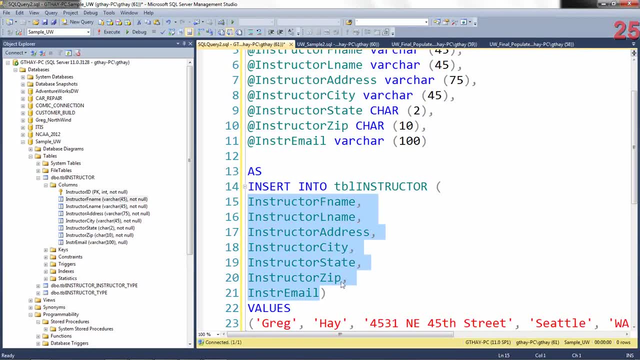 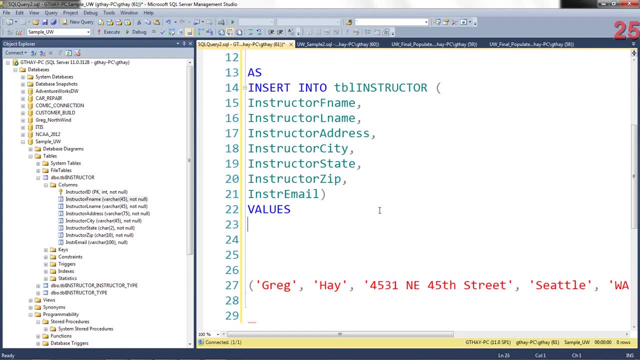 okay, we're good. now I'm going to insert into this table. we have these columns specified. now what do I do with values? well, let's do this. values will be: what do you think the first position will be? well, we're just going to call the first. 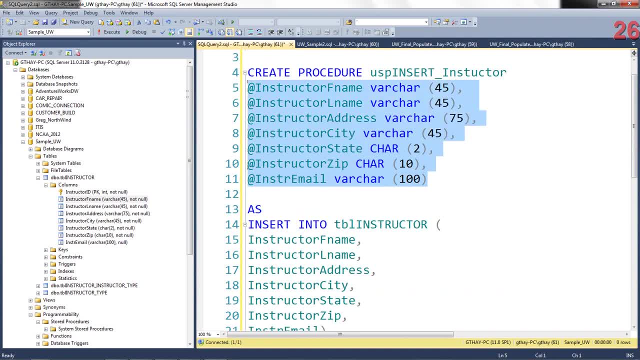 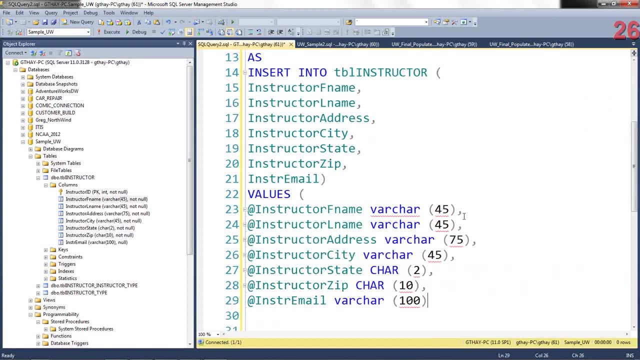 variable. I'm just going to do a little bit of sneakiness here. this is what it will look like. we actually don't need the table definition anymore, but the values are going to line up and this will probably become a little bit more obvious as we see it here in action. but this is how we process thousands and thousands and. 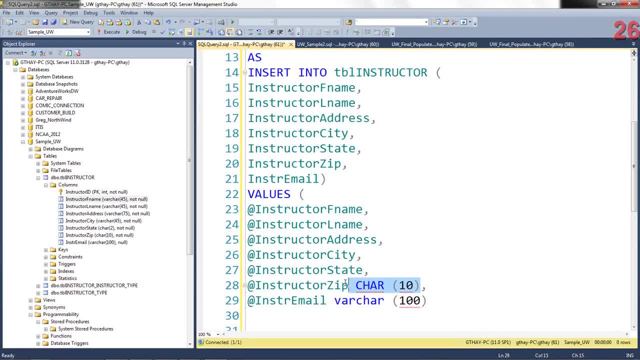 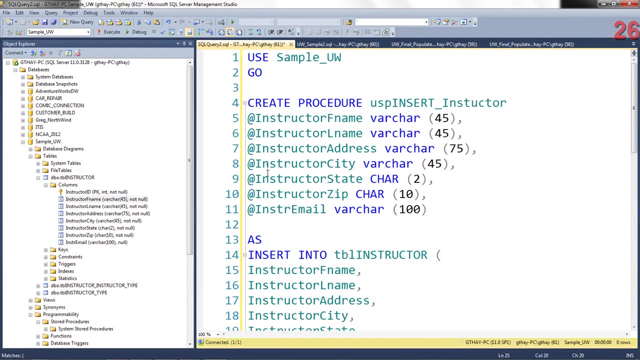 thousands of transactions every single day with stored procedures. now all we are telling the system is: whatever is in these boxes. whatever is in whatever is in the pizza box is: bring it in whatever is passed in. so we're the way this is. this store procedure is going to take one, two, three, four, five, six, seven, seven parameters. 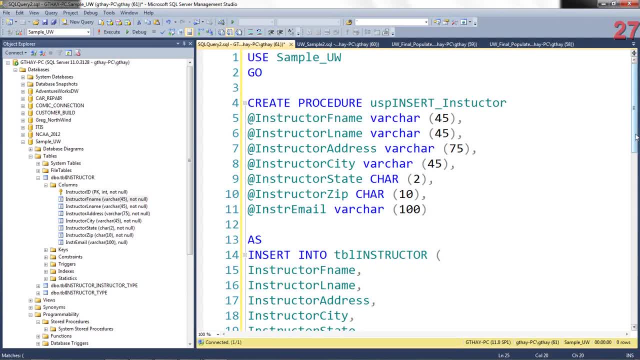 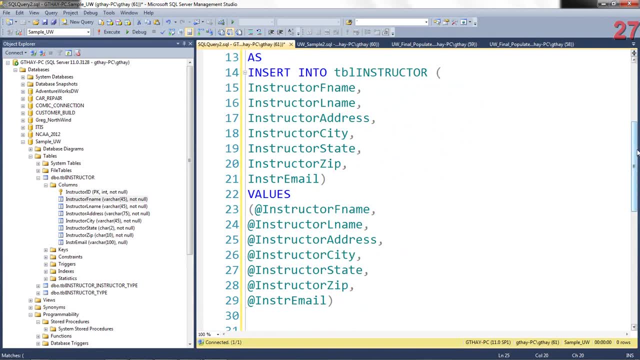 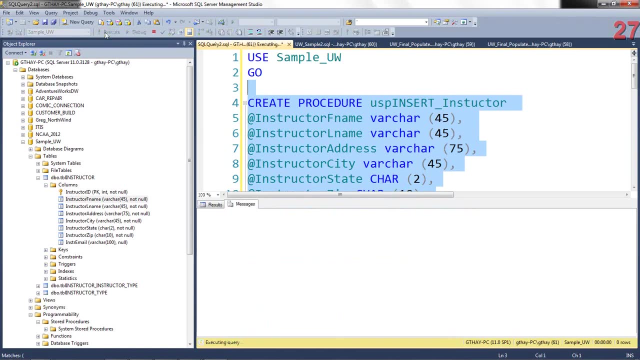 will be passed in. once those are in, they will be stuffed into the table. so we're not going to necessarily gain much if we're doing just one at a time by hand. we will gain an exceptional amount of just created it. we're going to gain an. 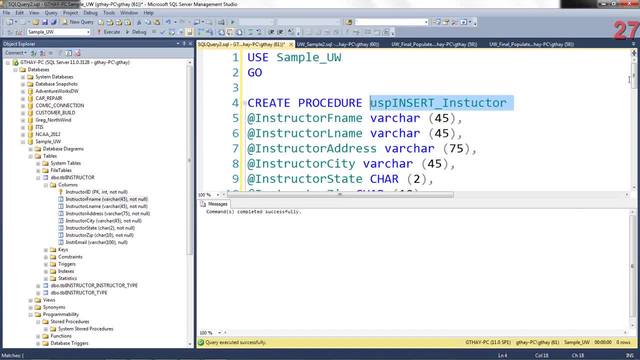 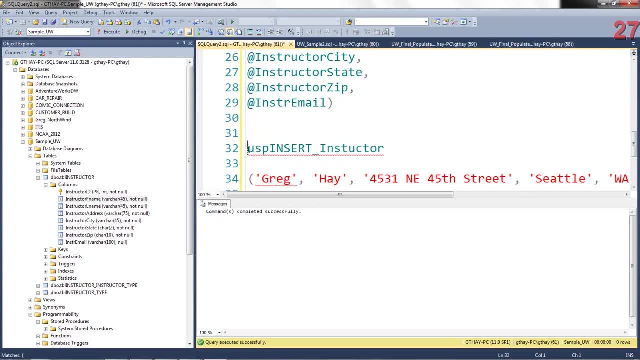 exceptional amount of flexibility and performance gain. when this is automated and we have it off the web form, we are going to execute this, we're going to pass in the parameters. know, since this data is already in its entirety, already in the day to base, let's, let's change some of this data so we have something. 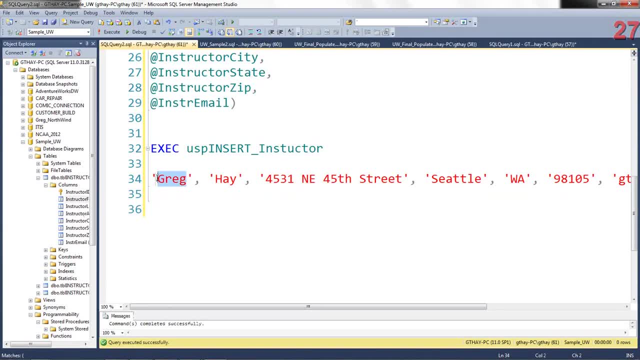 unique. what is? let's go. JP patches- JP. this was a clown that was here in Seattle way back in the day and when I was nine I was a patches pal. and when JP patches, the clown came to McDonald's in the U District, which is still there by. 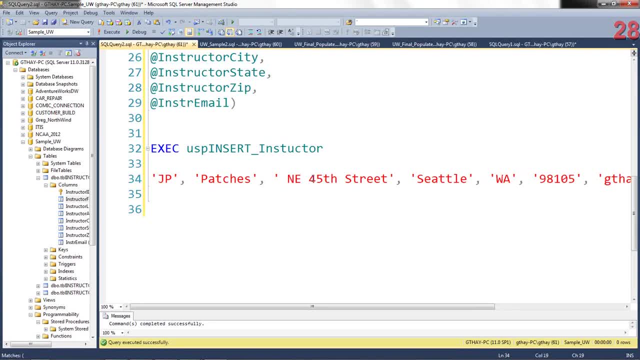 the way on 25th Avenue, not too far from the you. it was a huge deal. we waited in line, my brothers and I, for like two hours just to go shake hands with JP, which means nothing when it comes to start procedures. but I wanted to change. 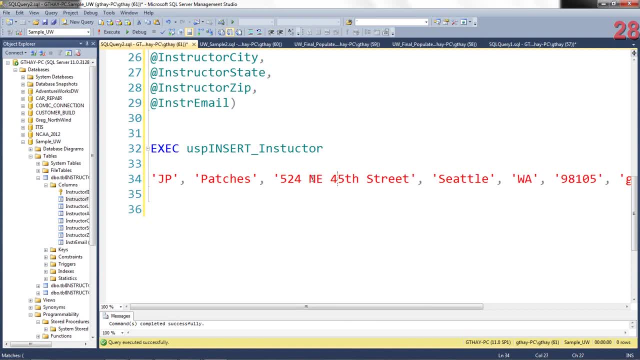 let's go northeast. let's go 25th Avenue Northeast. that's where the McDonald's is. 25th Avenue Northeast- that is in Seattle. that happens to be 98105. we need an email. JP patches at UW so see if I can move this over, just so we can see it. all, all we're. 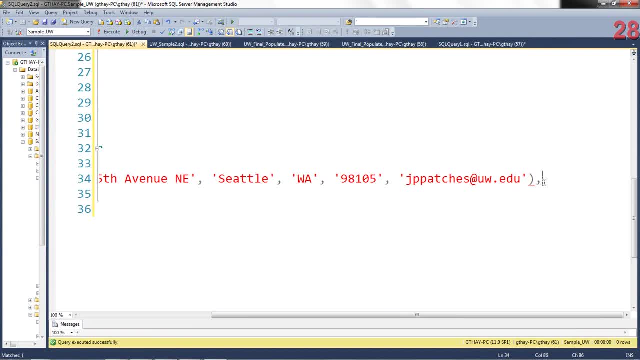 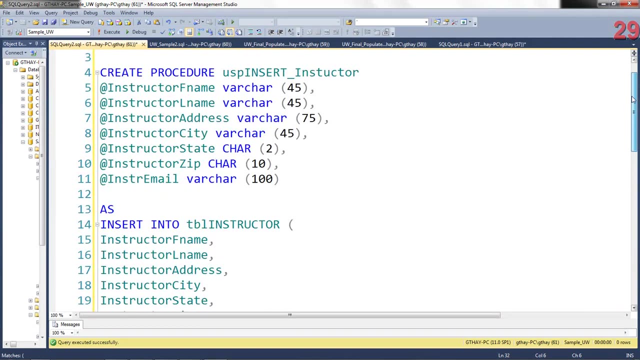 doing is now gonna call this story. I gotta get that last comma out. we're just calling and then actually I don't need that last little bit. we're calling this store procedure we just built. this code is now stored. it's gonna execute this code right here. it's an insert statement. it's taking in seven parameters. it is. 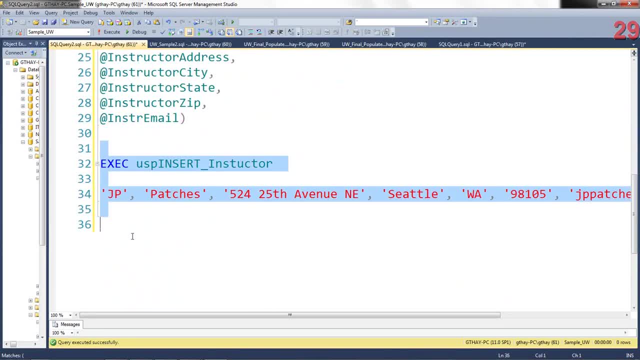 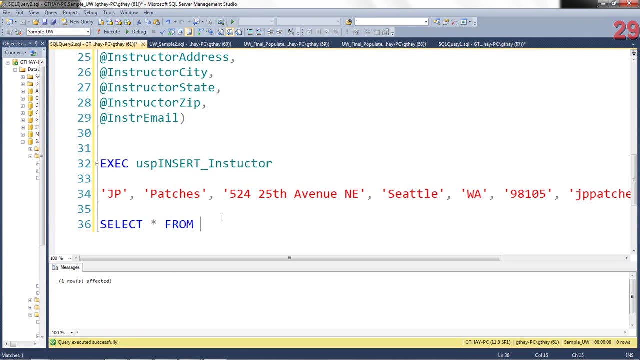 now created. I will execute this, but we have to pass in the values. I just executed this and it says one row affected. if we look at into the table now, select star from TPL instructor structure or we should see JP patches right here. we just entered that. 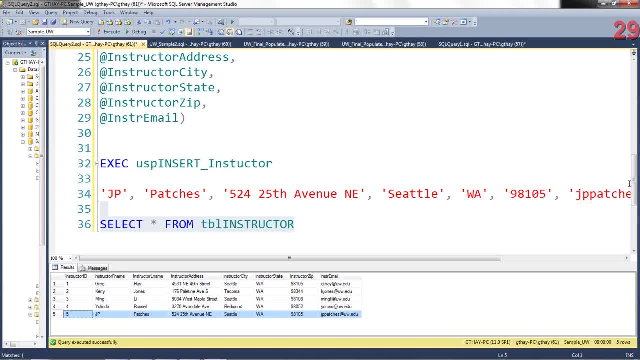 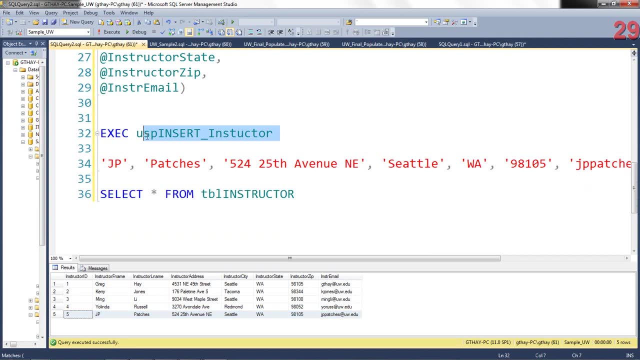 now all we do is hand code. these were not going to be gaining much, because I could probably write an insert statement just as effectively. where we gain incredible amounts of scalability is when this is automated off of a website and we have thousands and thousands of people- consumers- connected to a website. 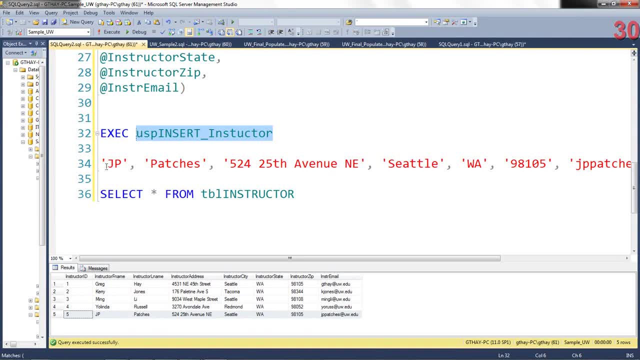 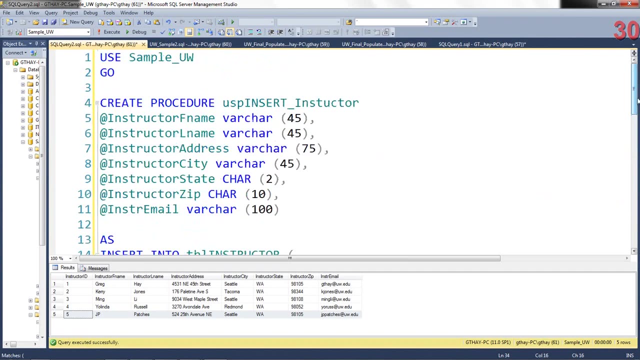 filling out the values themselves, signing up their own names and hitting submit. we don't have to have one person managing all of this. we kind of take it for granted, because we just assume that whenever we interact with the database that- oh, I had never really thought about it- that's how it's getting done, that's. 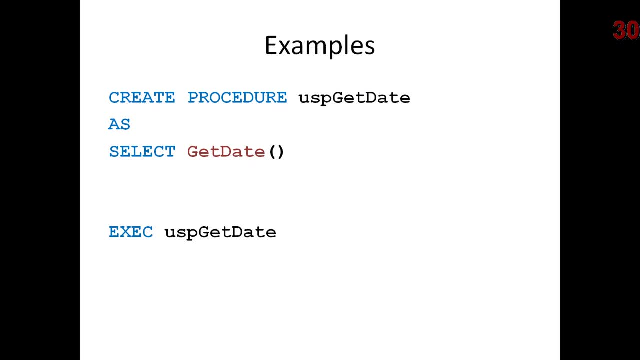 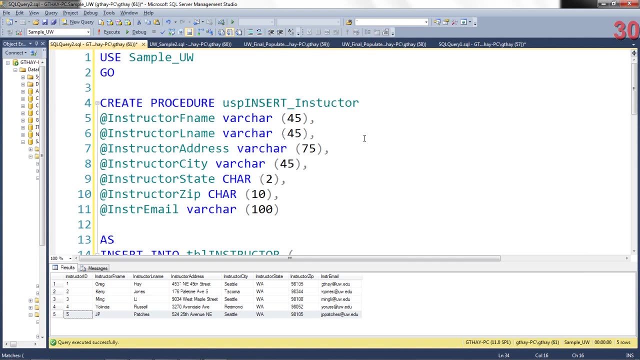 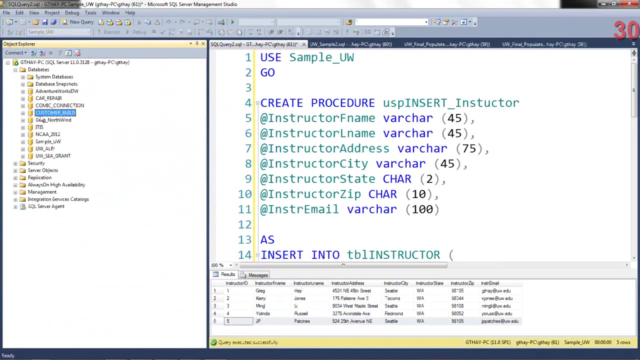 how we get an immense scalability. and again, a lot of insert, update and delete statements are done with store procedures. I want to show off another more complex store procedure. I want to show off another more complex store procedure. perhaps I use this in customer bill database store procedures. 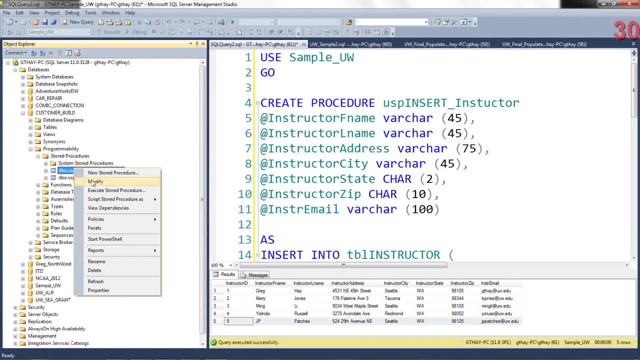 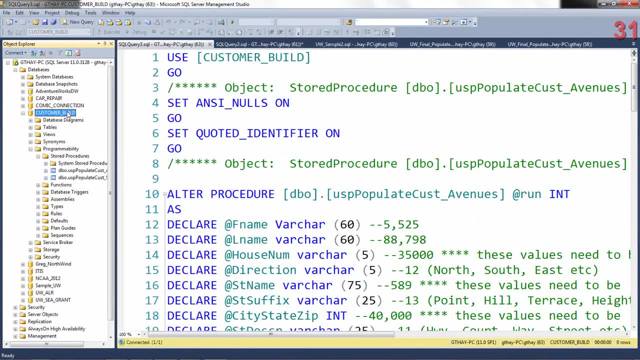 let's. I'm using this to populate a, so this database creates fake names- their real names- but they're assembled very quickly to create real looking names for testing. so I need to have, some times, 40 50,000 names of people with real addresses, real looking addresses. 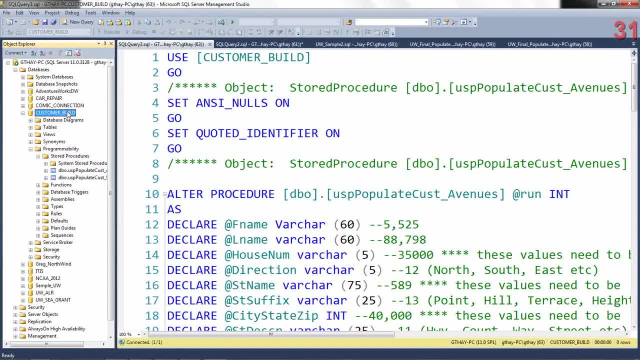 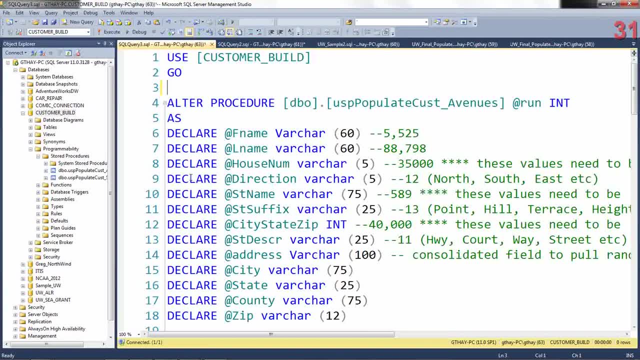 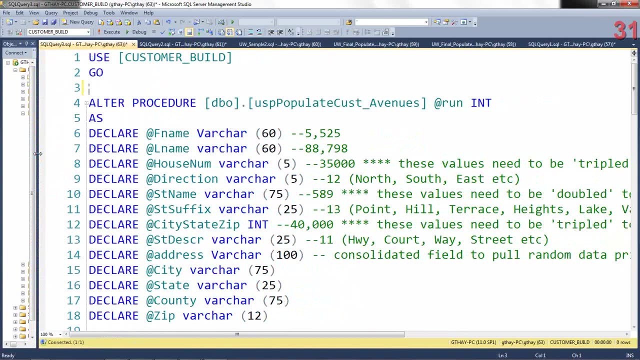 so I can do some transactions for testing purposes on databases. so I have this. I built this to specifically create fake names. I will show how this works. this just happens to be a little bit more complex and I want to show it off for comparative reasons. I want people to see that. okay, you can do a lot more. 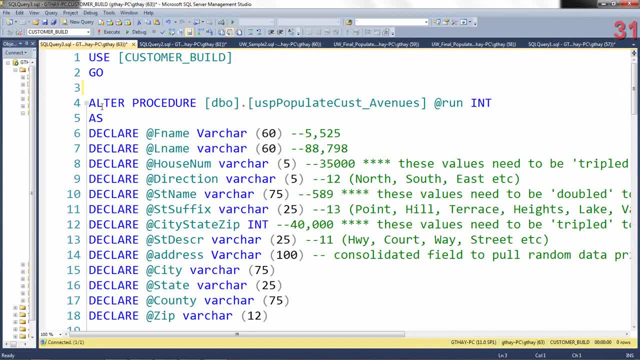 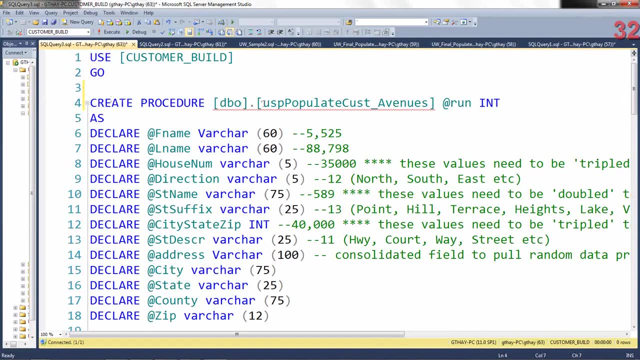 then do a single row insert. so let's take a closer look. this is listed as alter because the procedure is already been created. if we have not built it yet, say we want to put this in a different database, we would use a create statement. this is just some name USP. 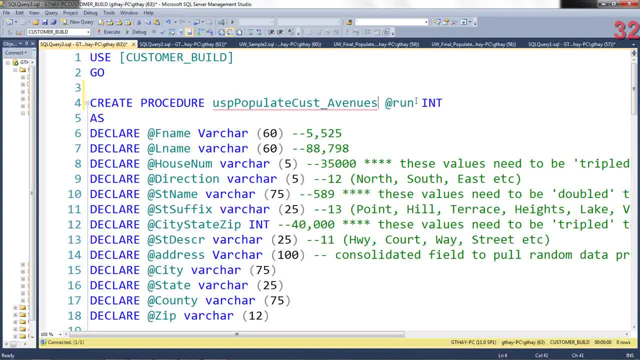 populate cussed avenues. I have one parameter. it is a. I'm calling that Ron. that could be anything. I could have called it Dave. what I'm trying to capture on the way in is just some digit, some number: five, five hundred, 40,000, the number of new. 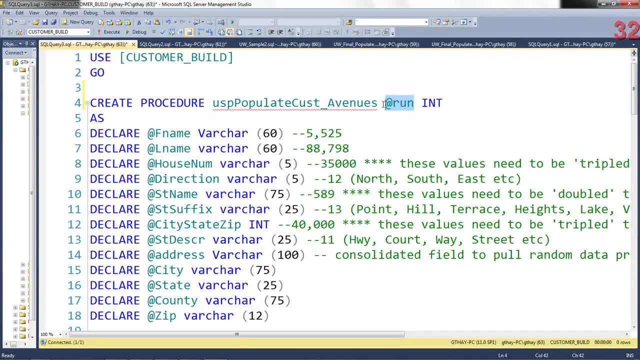 rose customers that I want created. so I need some number to just limit it so it doesn't run forever. put a number in it. put a number in it so it doesn't run forever. put a number in it and that's how many times it'll spit back new names or new numbers. 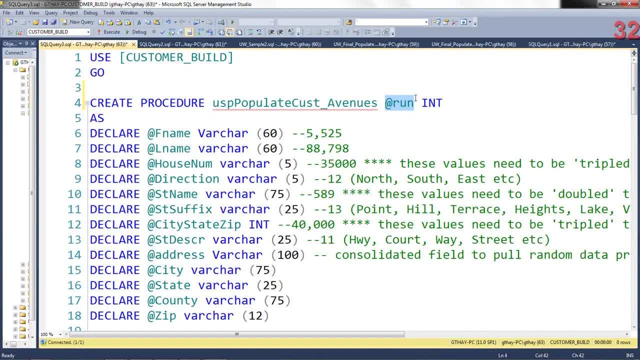 will go very quickly. we were already half an hour into this presentation, so I want to make sure we don't go on forever. that said, I mentioned that we have parameters. here's an example of a parameter. here are examples of variables. now they look the same. we have an at sign in front. we define a data type. 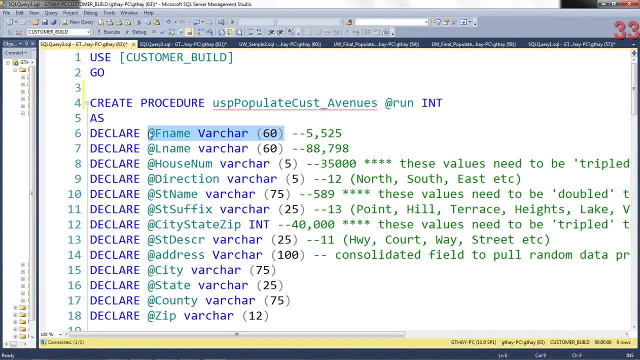 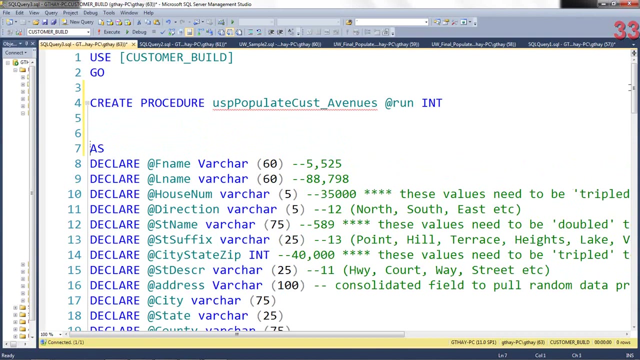 while we're doing kind of the same thing here, except we have to declare notice that it comes after the as, and then we declare a variable. these are pizza boxes and I'm calling laundry baskets inside the stored procedure because they occur after the as. what are these doing? 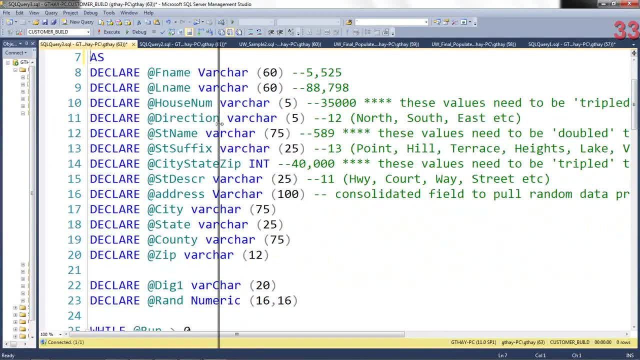 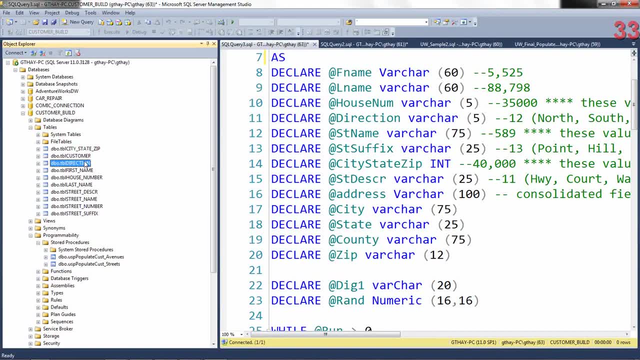 I have in customer build and I'll make this available on the class server. I have some tables I've assembled in these tables, various. I'll just show it off very quick. this will take three minutes. various tables that have random values that will help include: help build. 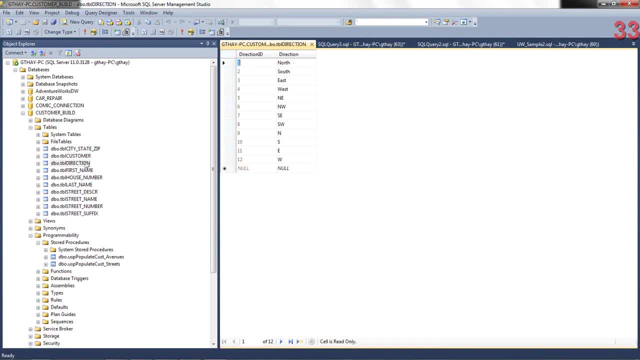 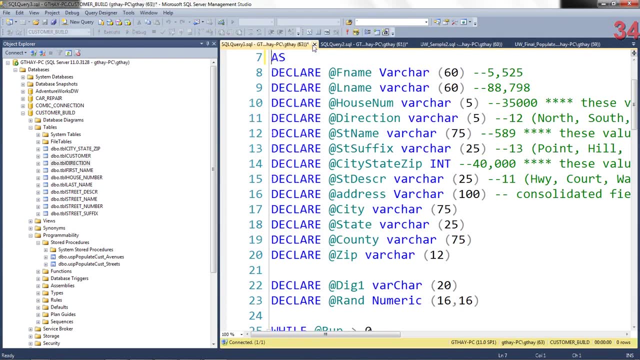 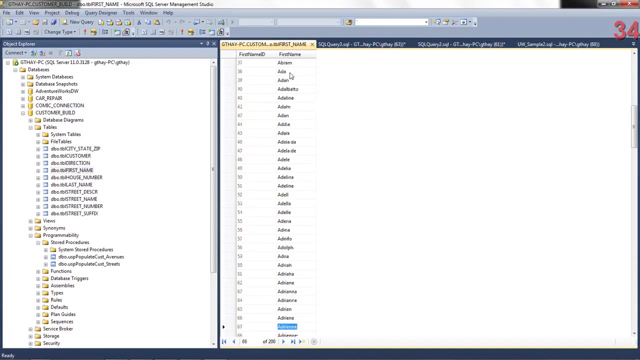 fake addresses. so we have in the direction table north, south, east, west, northeast, northwest, southeast and so on, and I'll be leveraging that data from the direction table when I'm building an address. you can imagine in the first name table I have some large number- five thousand- first names. 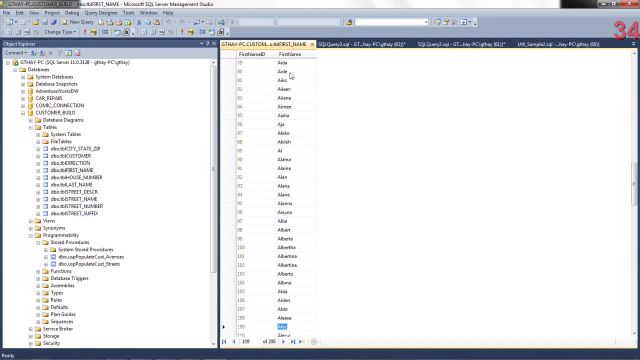 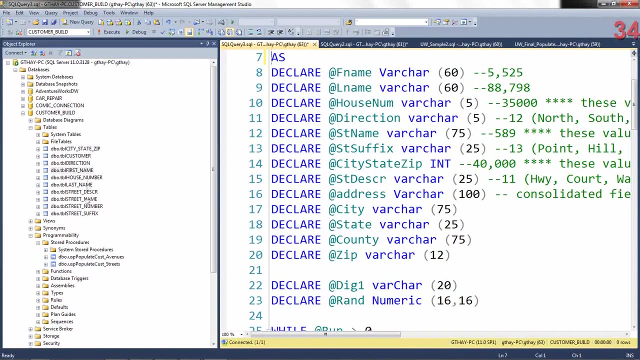 five thousand first names. these are all legitimate. I pulled them right off the internet. pick your random name: Alina, Aline, Alicia- those are random first names. I do the same thing. that we don't have to go in and take a look at the same thing for last names. 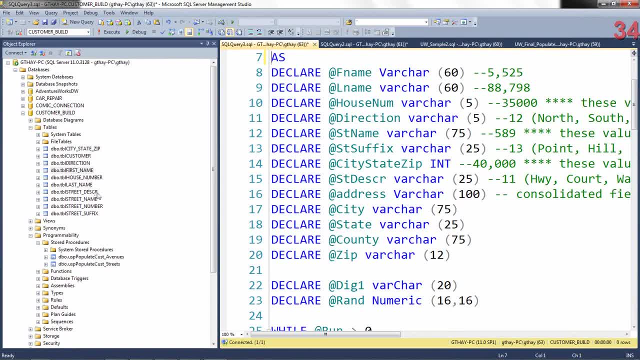 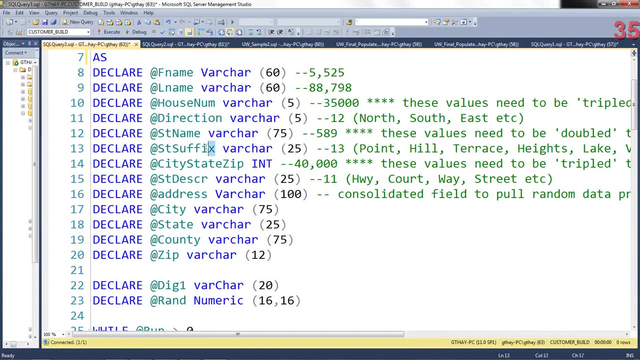 street descriptions, so it's like court Boulevard Avenue. I'm blanking out what they were: circle right way, view drive. all of these are different ways to construct an address. they live in their own tables. that said, I'm going to go out and pull one value from each one of these tables. 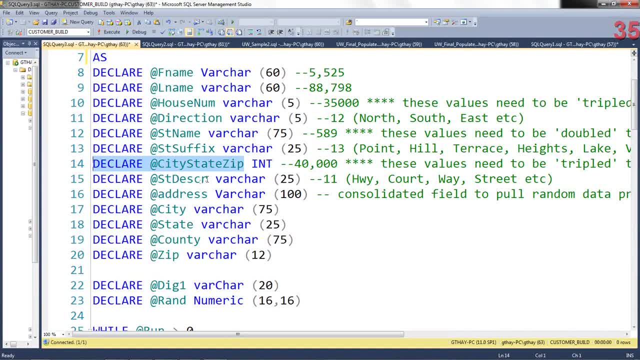 and construct a reasonable looking new address. by the way, I did look up the actual counties, the actual zip codes of something like I'm going to guess forty thousand. I put in over forty thousand cities. you wouldn't think there's forty thousand cities in the United States. there is. 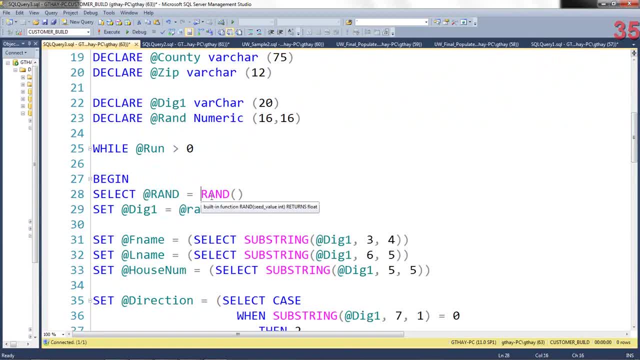 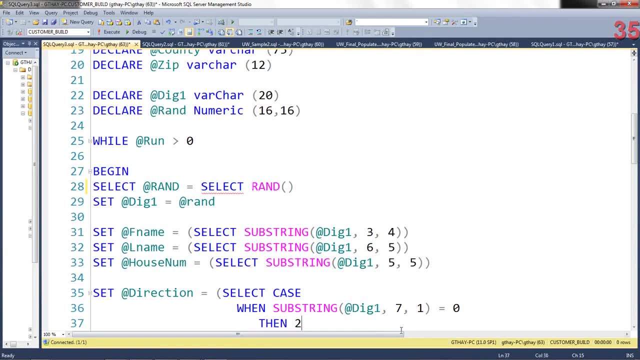 we have a function here. I may have showed this off in a previous lecture: select rand. what is select rand? do wallet creates a random. if I can get this to, what am I? how come that's? that's not going up. it creates a random. I want to show off the results screen. 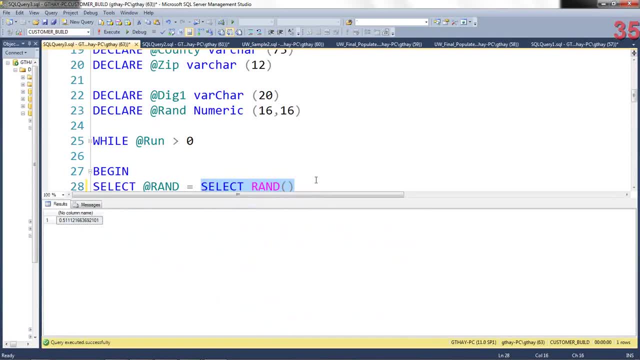 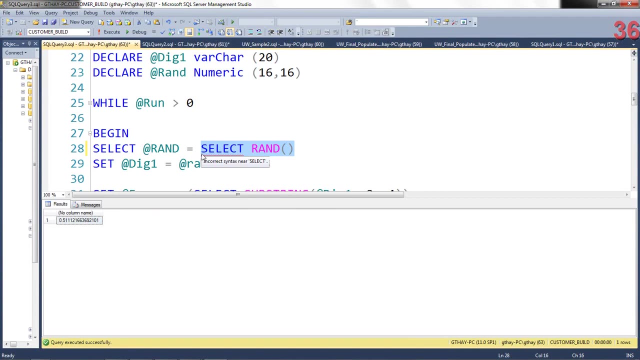 we'll see what we can get there. there we go. once I execute rand, what does it do? it just generates a random number. notice right down here: zero dot five, one, one, one, two, one. don't know if we can make that any larger. I issue it again and this always changes. you know, just literally a very, very large number: sixteen days. 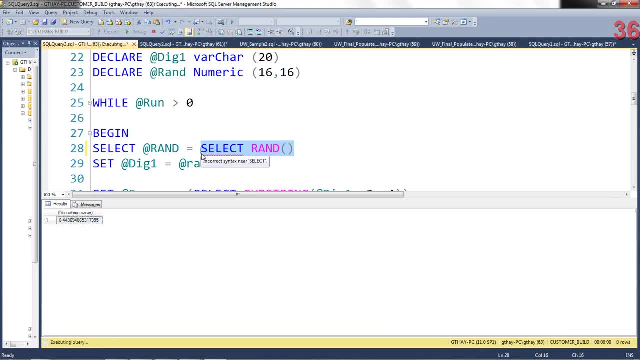 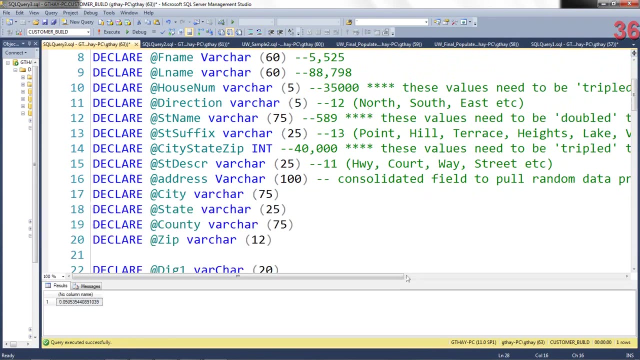 digits long. that's going to generate a random number each time it's executed. okay, why do I want to do that? well, I want to capture random values because I want to build a random, a random set of addresses and I'm going to jump into each one of these tables. I get a random first name, random last name, random house. 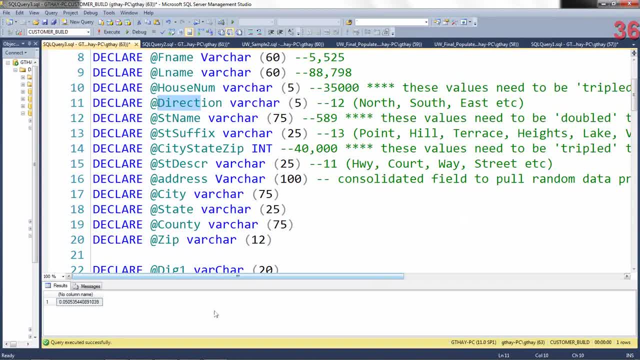 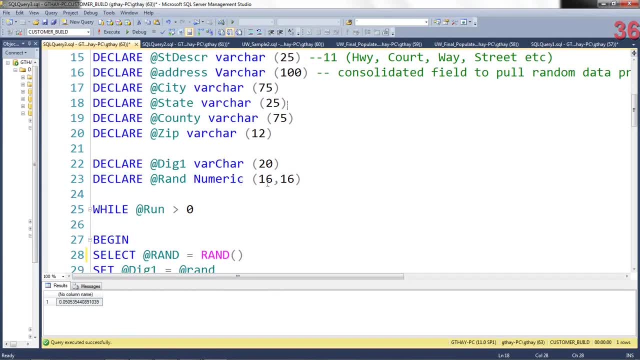 number, random direction, all that based on a random number. okay, and I don't want to spend, you know, 30 minutes, I can. you know I can talk forever about this. sometimes it gets kind of boring. I issue the rand function and then I capture the value. I said these are laundry baskets. sometimes we have to capture and move. 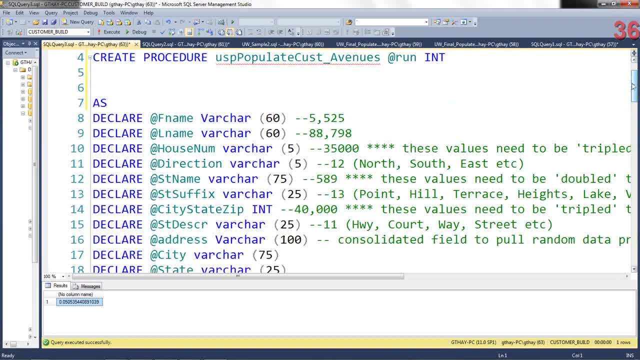 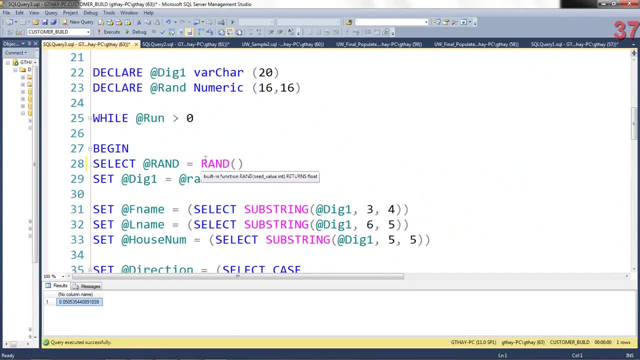 data internal to the stored procedure. this is an example. we capture a value. we first create a value, random function, 16 digits. capture it, I shove it into a laundry basket right here, so I'll explain this. remember the number that we passed in in the parameter at the very. 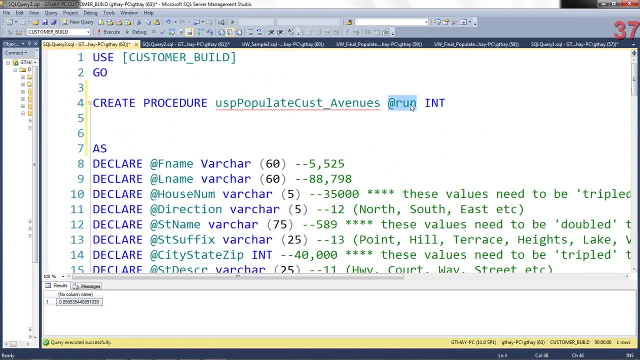 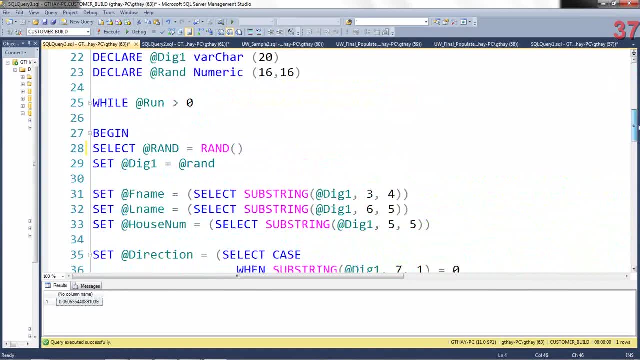 very, very beginning. this is some number. this is how many rows I want belt. it could be five, it could be 7500. whatever it is, we're going to say tell you what, while that number is greater than zero, do something. well, we're going to move laundry around, we're going to move some data around. we're. 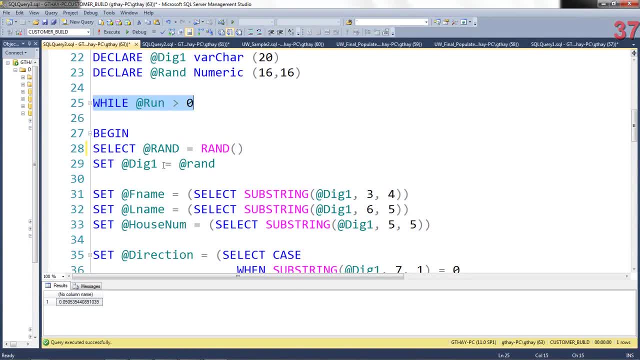 going to construct an address each cycle, so we're going to cycle through this quite a bit. now the rand function: here it comes out as 16 digits. for whatever reason, I cannot throw that directly into a variable character string. I have to first throw it into a numeric string. so the first laundry basket this data gets. 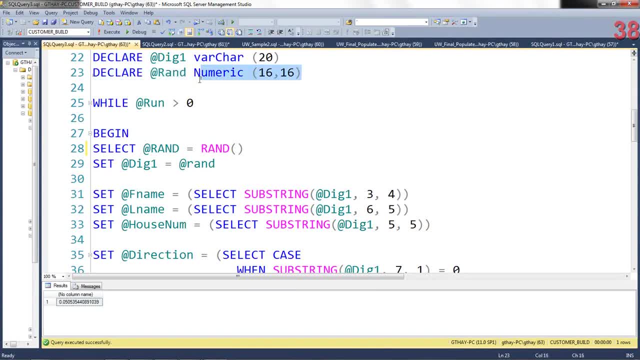 chucked into is going to be numeric, it's going to be defined as numeric. then, immediately after I chuck it right here, I chuck it into this laundry basket, rand at rand, it's numeric. I immediately copy it into a variable character. why do I need to do that? well, I. 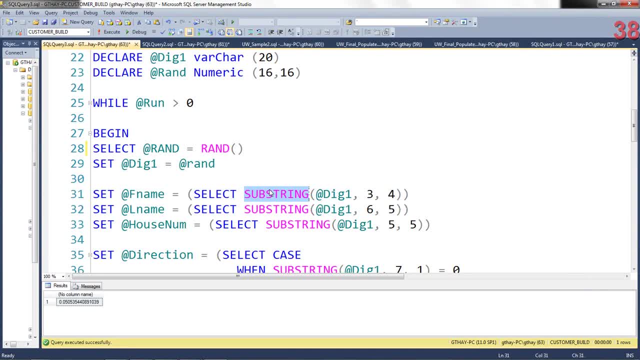 want to work a few extra. I want to climb into that laundry basket and pull out only the digits that I want, and I cannot do that with a numeric. with a numeric that defined as numeric, I can only do it if it's a character string. so not to. 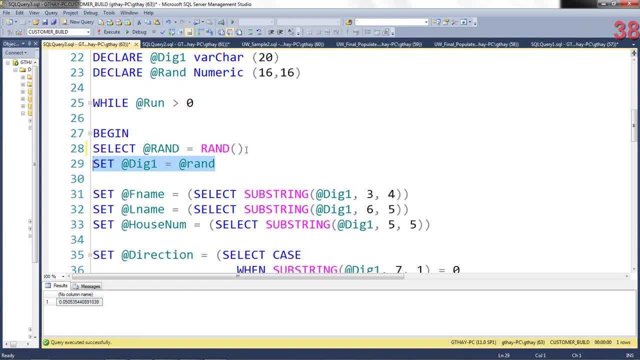 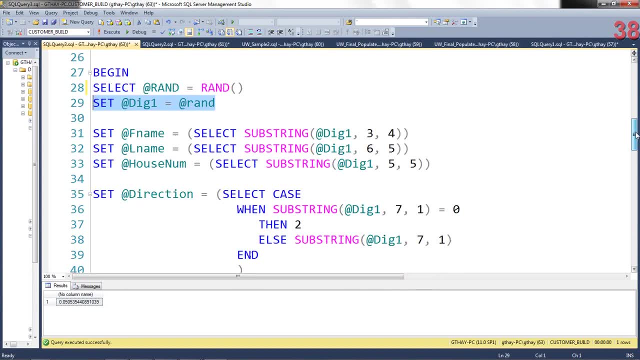 get too detailed. we have a couple laundry baskets here. we just sorting laundry, which is funny because if you talk to my, anyone in my family be like you sorting laundry. what are you talking about? never happens. moving on, we have first name. that was a variable. we're going to set that to something. we're. 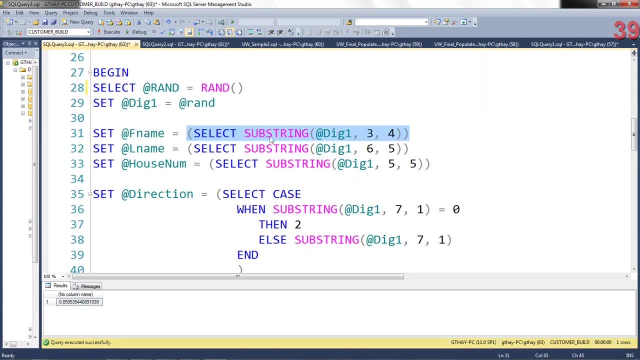 going to do a select statement. remember when I said I wanted to get into a another laundry. I'm going to pick a random laundry basket, we're going to put a survey in there, so let's go into a neePoint rule, and we're going to createاءúu an errorl phone number which basically sums up that line. if someone did you to that line and your statement will say: bearer washing all dishes for your SG line. 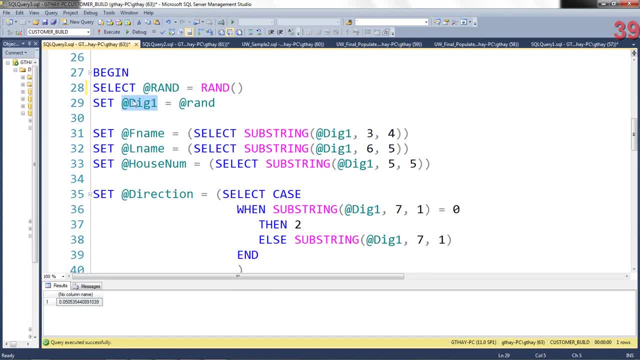 another laundry basket. This one's going to be character based. I call it dig one digit one. whatever, I'm going to look into that 16 digit value right here. This is 16 digits in the dig one laundry basket. I'm telling it with a substring function to go to position. 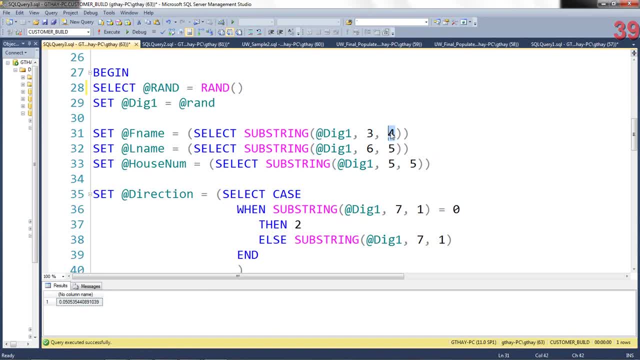 three and give me the next four digits. Well, what is position one? Position one is a zero. Position two is a dot. Position three is also a zero. I don't know if we can see that here. It's a little bit small. Let's see if I can capture that. This is what is in the 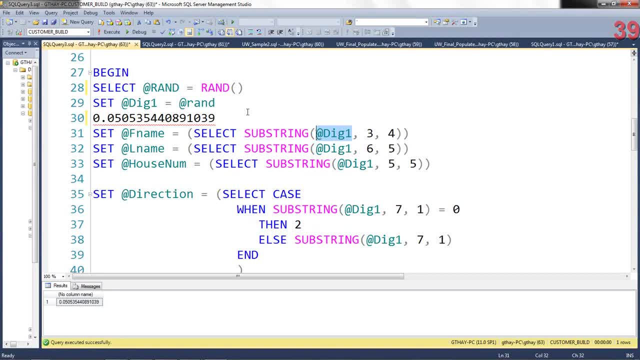 what I'm calling a pizza box, the at dig one. I want to go to position three. There's position one, The dot is position two. It won't. let me highlight it. Position three is actually the number zero. I want the next four digits, beginning with position three. All of a sudden, 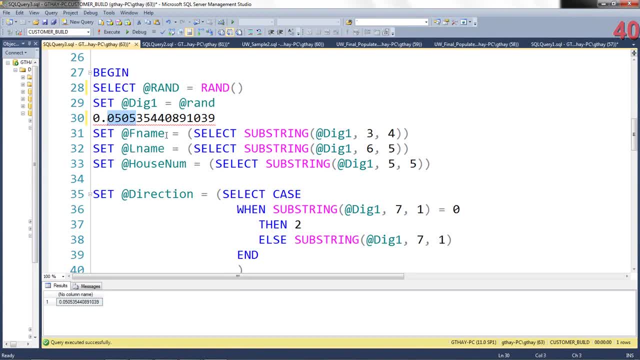 at fname is now populated. It's a laundry basket. It now has a value of 0505.. The last name is now going to go to position six. One, two, three, four, five, six. It's right here. 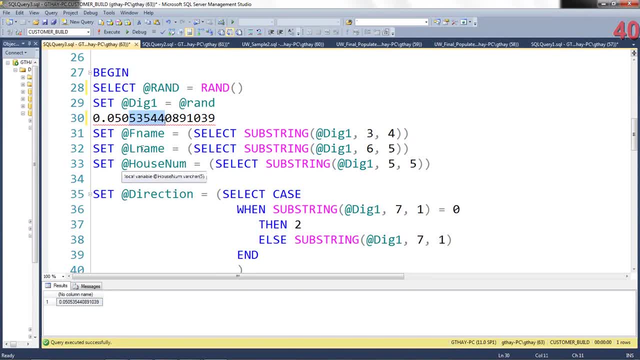 It's going to go five digits. The value for last name is going to go to position six. One, two, three, four, five, six, It's right here. It's going to go five digits. The value for last name is going to. 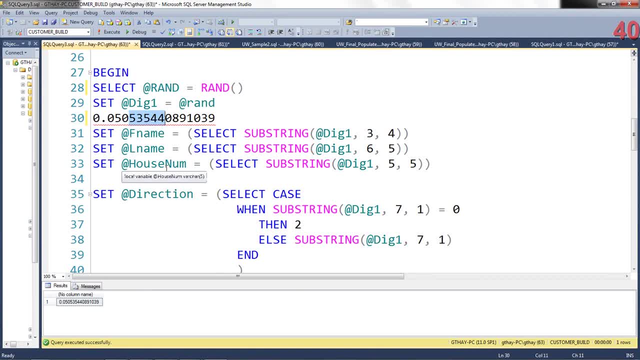 go five digits. It's five, three, five, four, four. Why am I doing this? Well, what I want to do is then go off and populate these again. If I call these values that I'm first putting in here the primary key values, then when I go down to construct all the way down here, 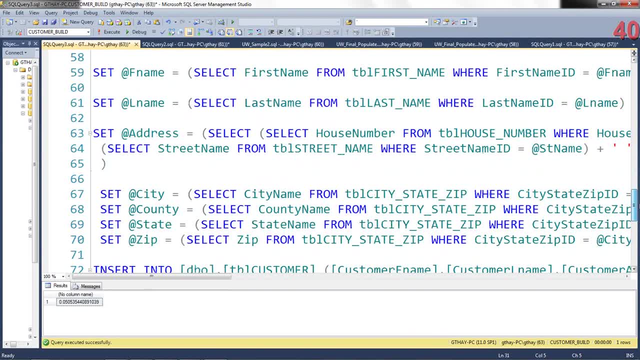 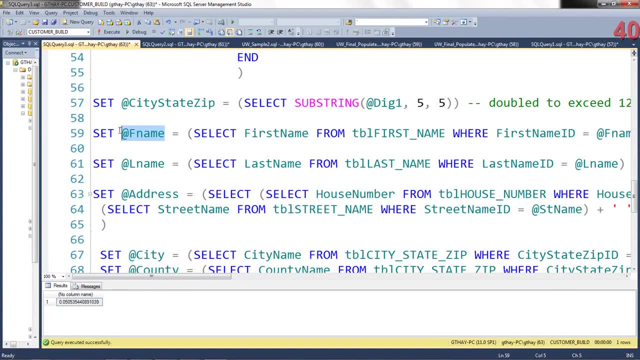 – remember, this is one stored procedure. When it comes time to building and getting an actual first name like Alina or Alicia, well, I'm going to leverage what was in the first name. go out to the first name table. remember there's like 40,000 names. 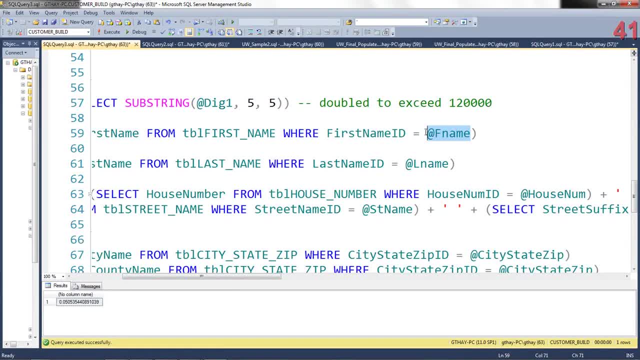 out there and where we have, I want the primary key. in this case, first name ID is a primary key where it happens to equal whatever it was for the first name: five, zero, five, zero, five. so I'm basically looking up the first name. give me the first name ID. I'm sorry, we're looking for the name right here. I'm. 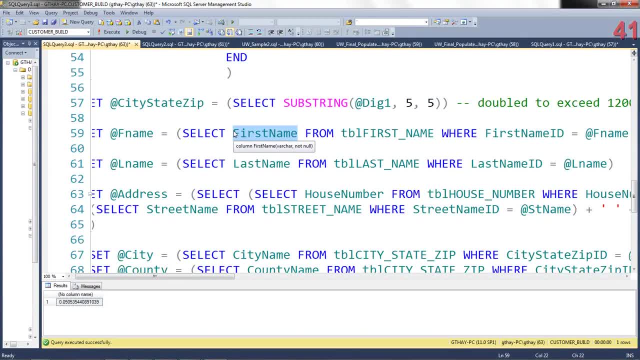 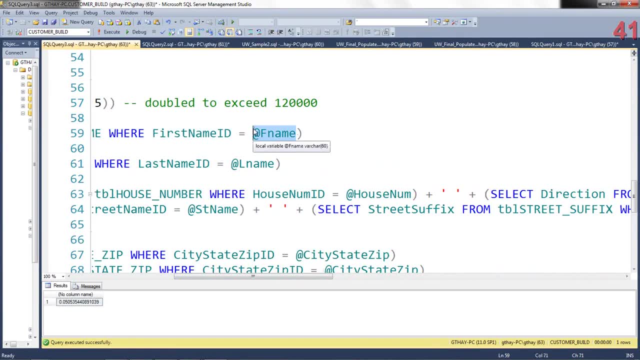 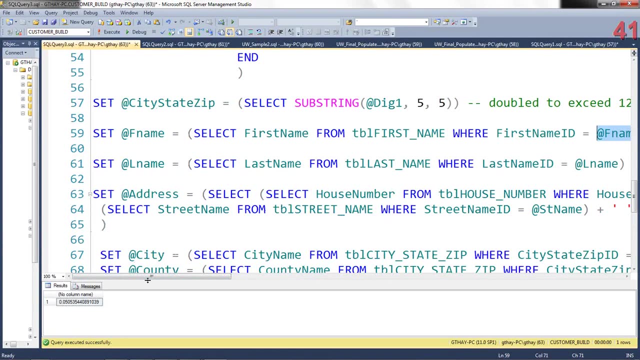 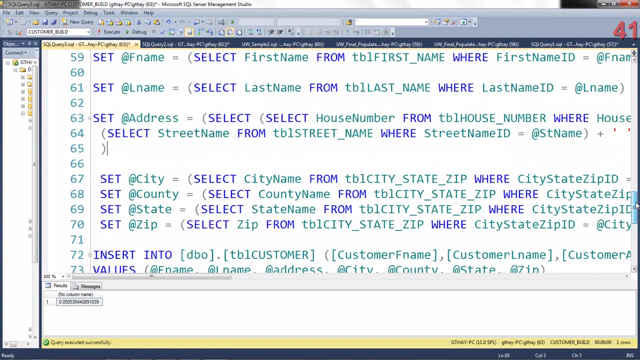 capturing the name. I'm pulling the name Alina if the ID value happens to equal whatever was generated in the random function. not rocket science, somewhat clever, probably more work than needed to be done just to create a store procedure that's going to give us a fake list of names. well, it works out well when we do. 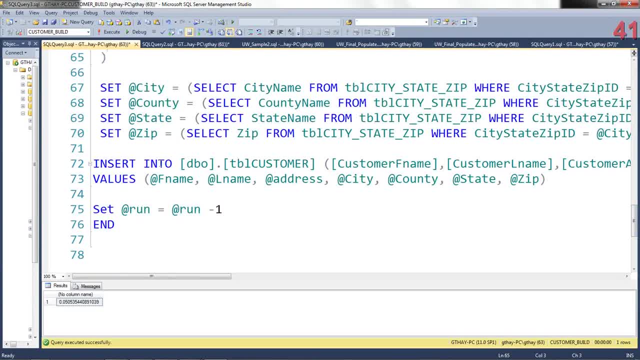 like ten thousand at a time at the very end. you can see here I'm doing in insert statement. these originally were digits. then I ran a select statement and repopulated them so these: this laundry basket is being used twice. once to get a digits set of digits, then it's going to be a name that was populated based on. 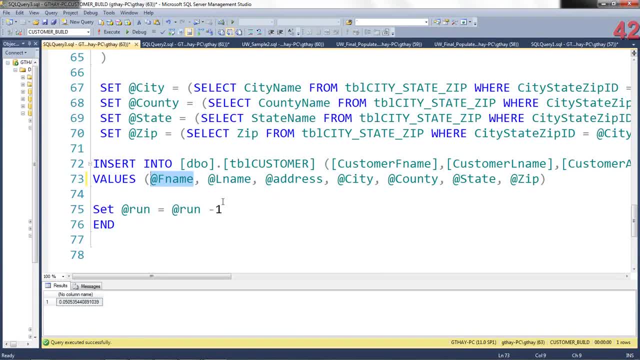 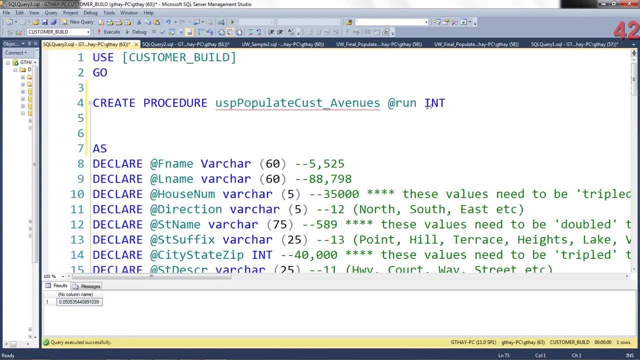 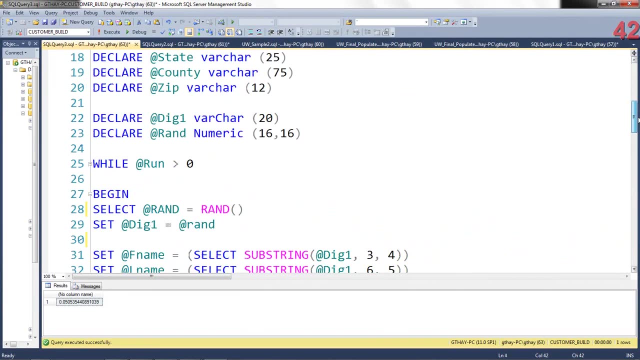 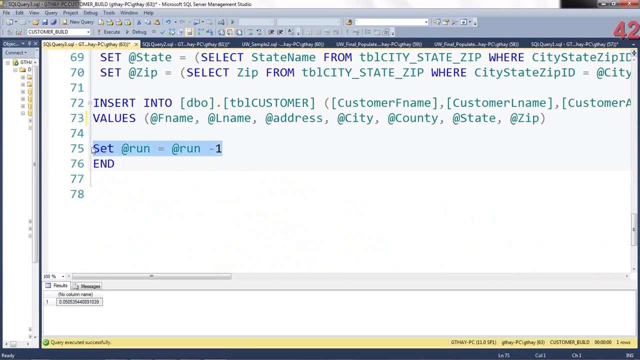 what the digit values were. and then I decrement my parameter. remember again going to the very top. the parameter was the number of rows that I wanted this to run. we're doing a while loop and if we don't minus this eventually, it will never get to zero. vice said it. 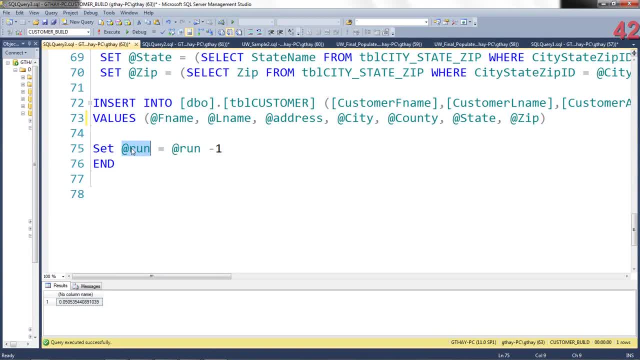 let's say I passed in the numbers 75. well, set this parameter to what it used to be, minus one. now it becomes 74. it runs and does another random function, does a whole nother artificial name creation in searches into the table. then comes here again and we go: well it was. 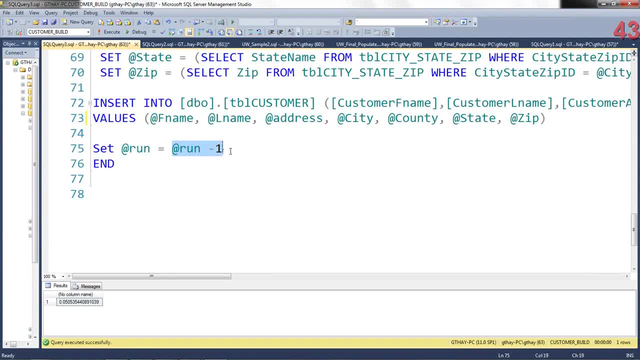 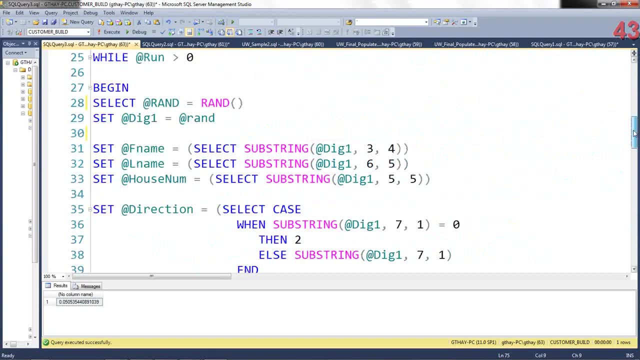 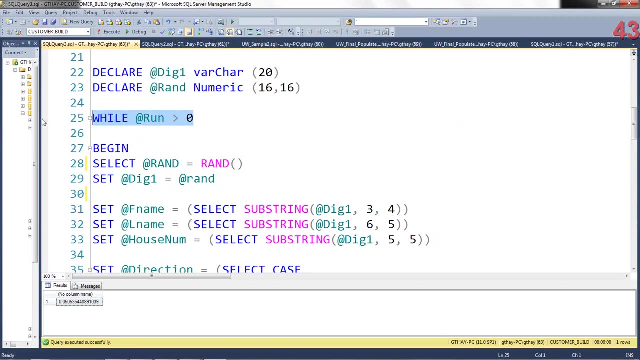 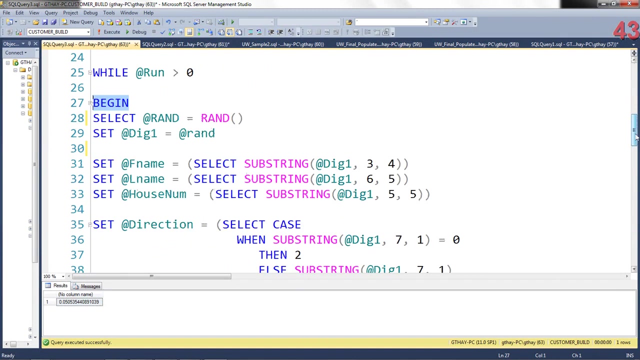 74. now make it 74 minus one. ok, now it's 73. then we run the loop again. eventually it gets down to zero and since I have a while loop right here that says, while that number is greater than one, begin and do this code. so this is called a while loop and we run the code that many times I wanted to. 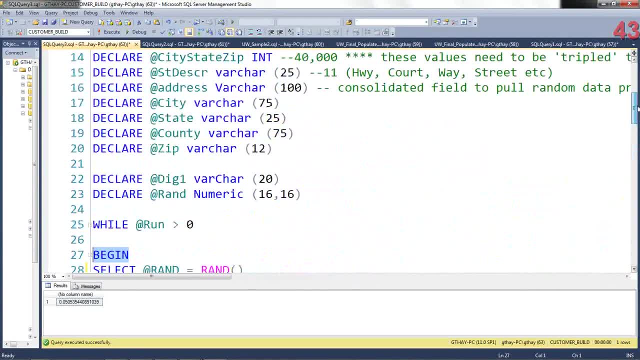 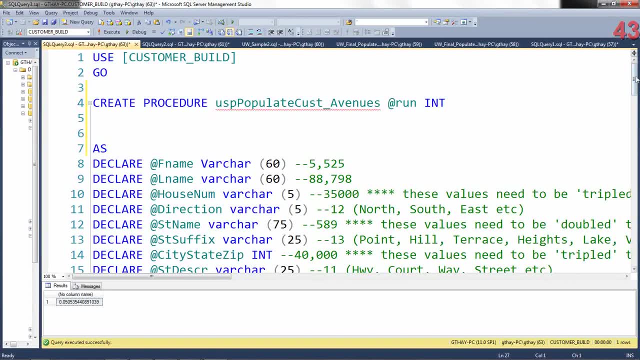 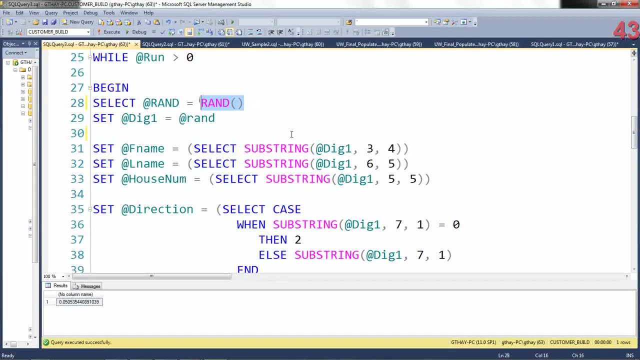 show off a couple examples of how a stored procedure is more than just doing a single row insert. it can be relatively complex. i'm going to argue. this store procedure I just showed off is not too complex. it has a couple interesting things going on, with a random function, a while loop, some substrings going on. 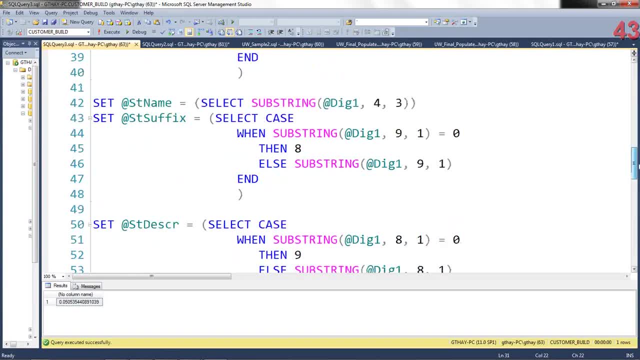 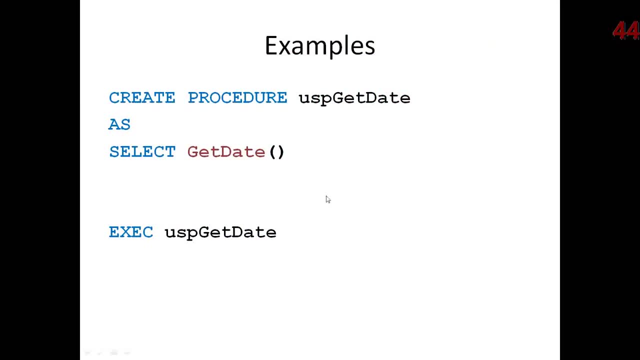 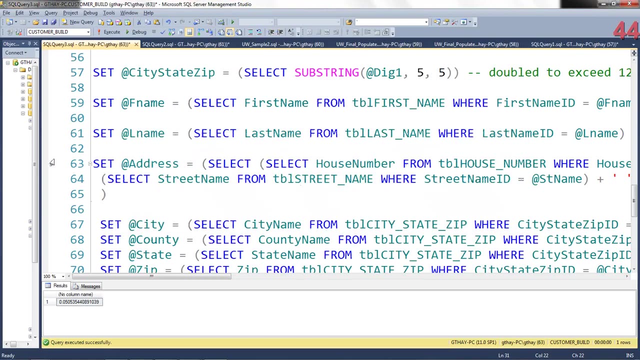 that's not going to work for me. it's not too uncommon and eventually it populates a table with a random set of values that I can then use when I populate. let's just go one more time. already already explained what it is. it's take a look at what it does. 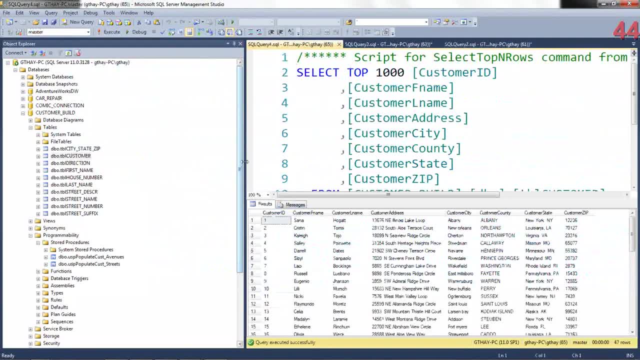 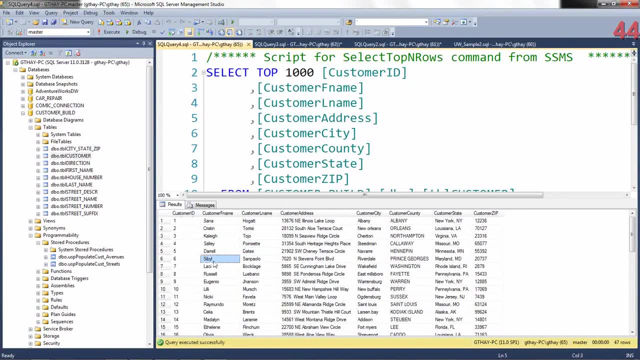 stuffs data into here. you can see that this may or may not look like. you know we have real names here. Daryl dates civil. Sen Paulo great will constructs a random street address in a city that actually exists. if you go to steedman, Missouri, it is actually in Missouri and 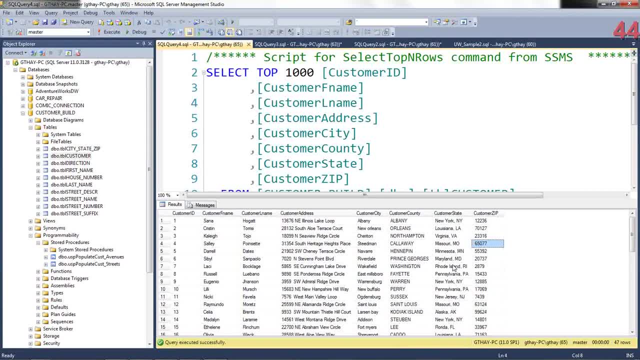 this is actually the zip code. I was able to get this from the internet, so this is real enough looking that when we run transactions as a proof of concept in any new database it doesn't look like junk data. it is very distracting sometimes when we see bla, bla, bla bla, stupid junk drive some City, USA and people get confused, or they. 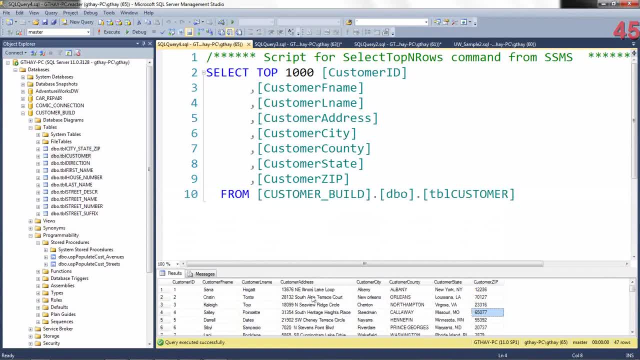 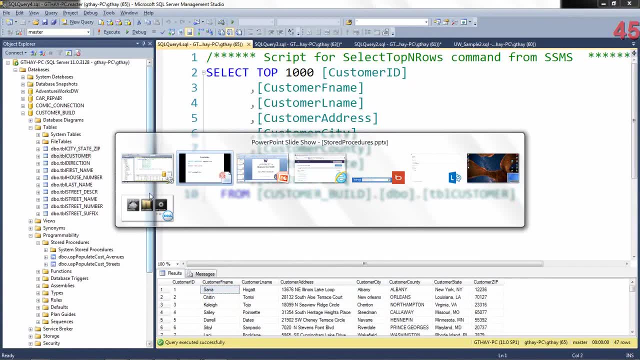 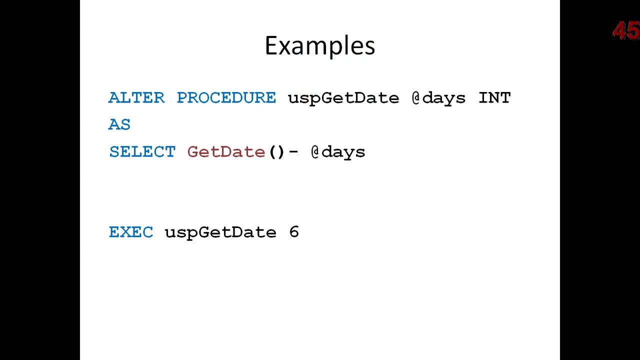 get distracted by the fact that the data doesn't look real. once we do this, people look out and say, hey, it looks like you already have data working. not really, it just puts us in position to make it look better. moving on, showed off how we can take the procedure and add a parameter and that and then 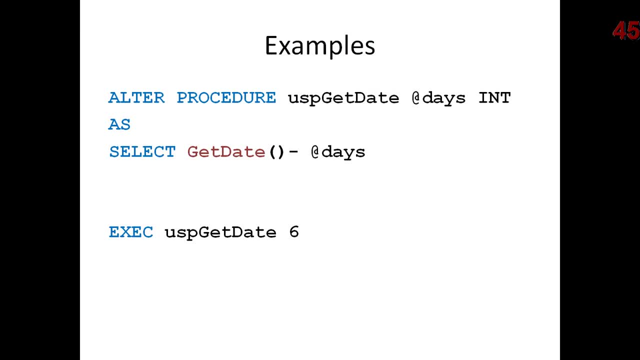 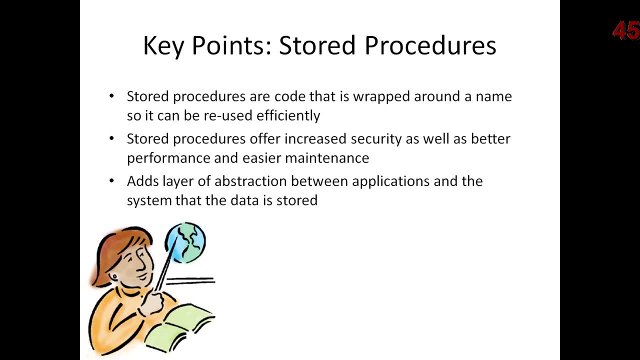 reference that parameter when we call that store procedure. so again, key points. a store procedure is a set of code, that's all it is. it has a name. we can reuse it many, many, many times. some store procedures get called millions of times every day. authentication to hotmail is a billion times a day- very, very large.